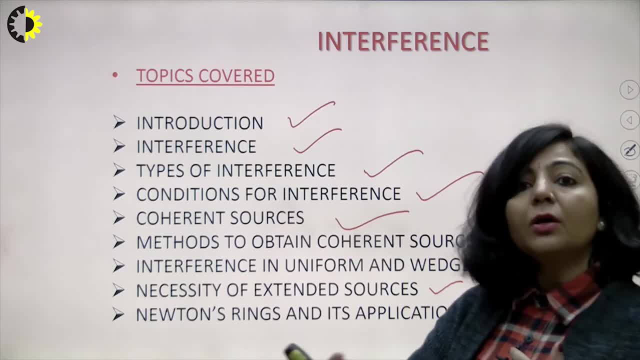 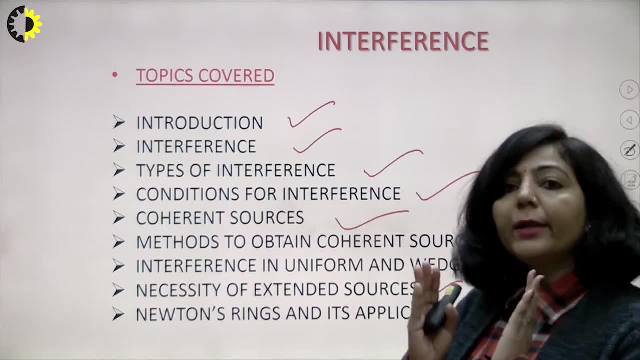 entire thin film at one time or at in a single go, then always an extended source of light is preferred, Whereas if you are using a point source, then you can see only a small part of the thin film. So that is the reason: extended sources. 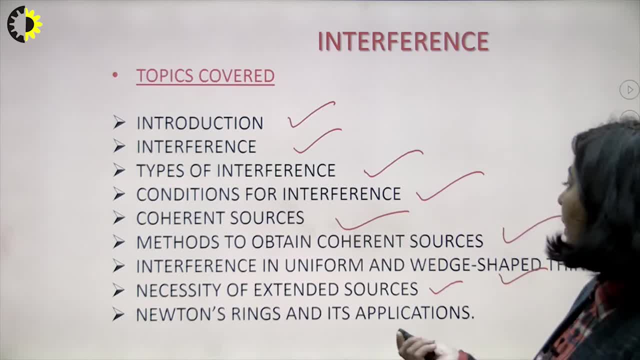 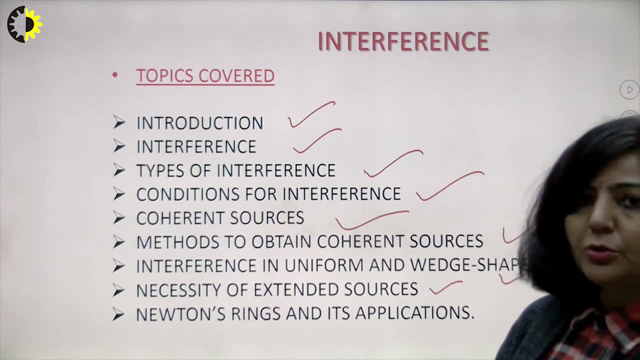 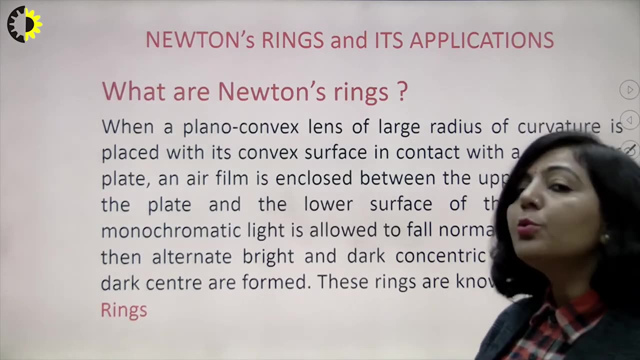 of light. they are always preferred over point sources. Now, the next topic which today I am going to discuss, that is Newton ring experiment, and we will also discuss some applications of this experiment. So now, the first question which comes to our mind when I am saying Newton ring experiment that what are Newton rings? 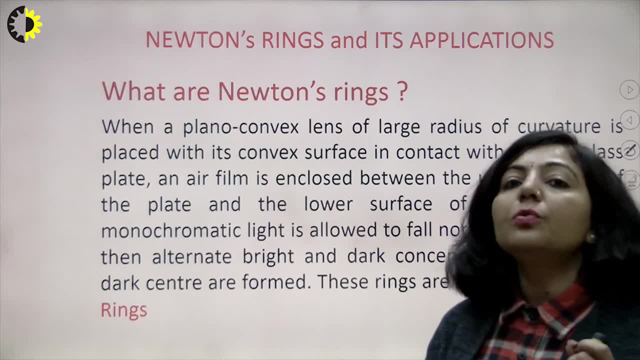 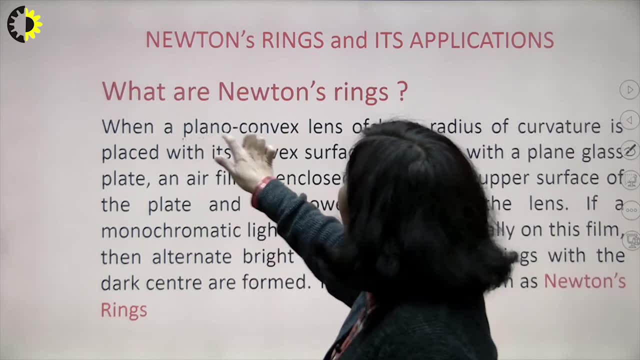 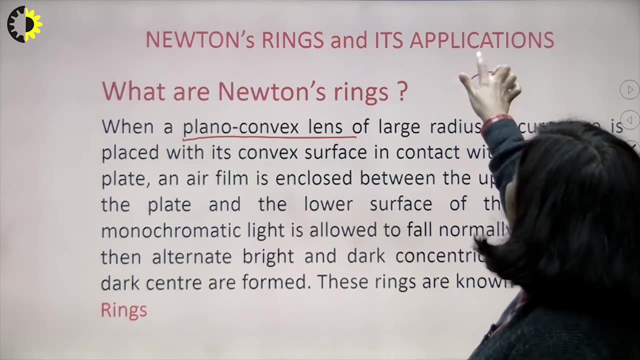 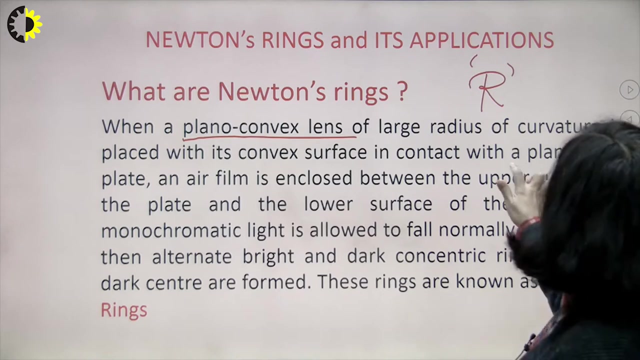 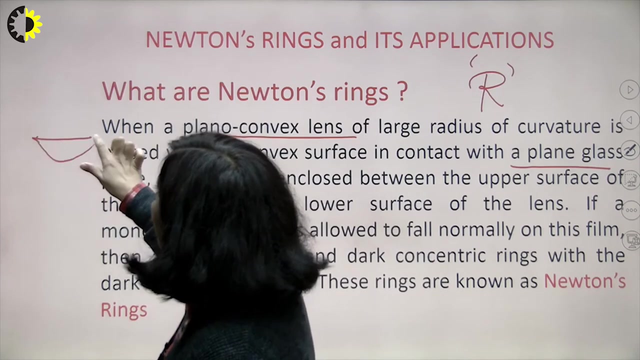 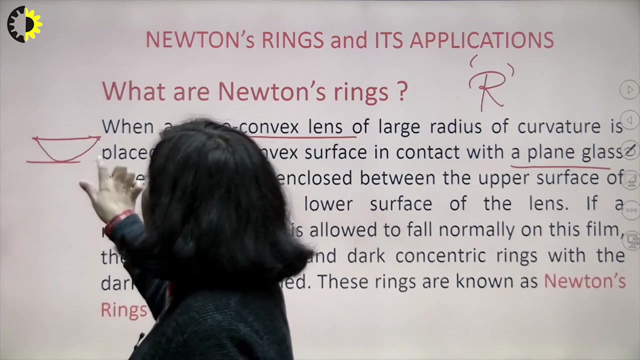 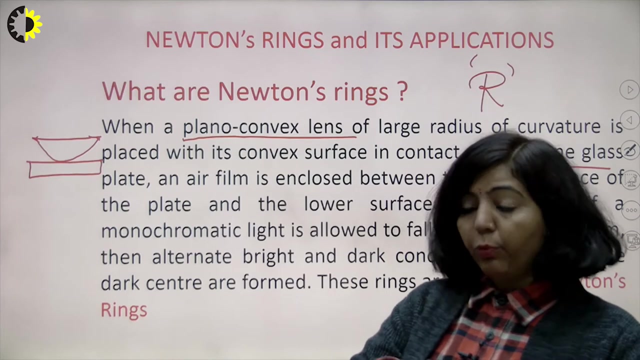 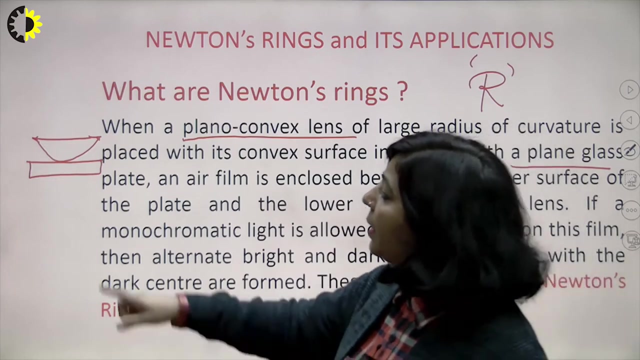 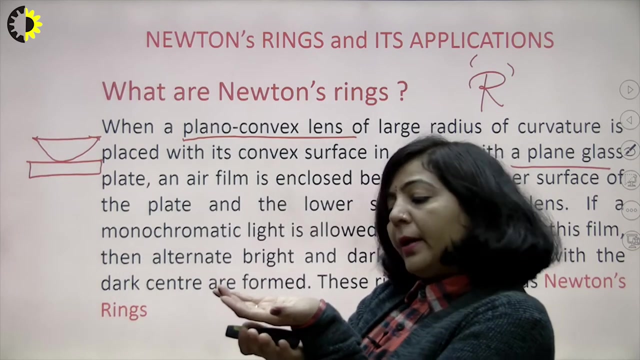 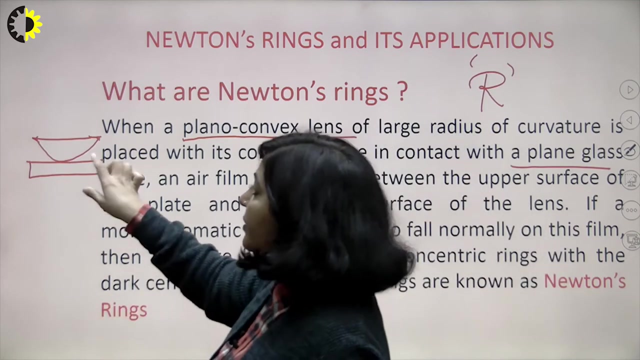 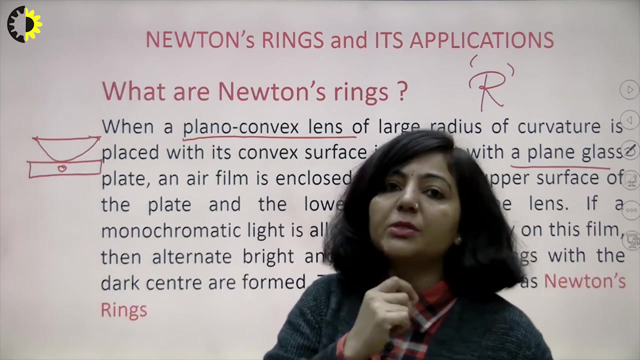 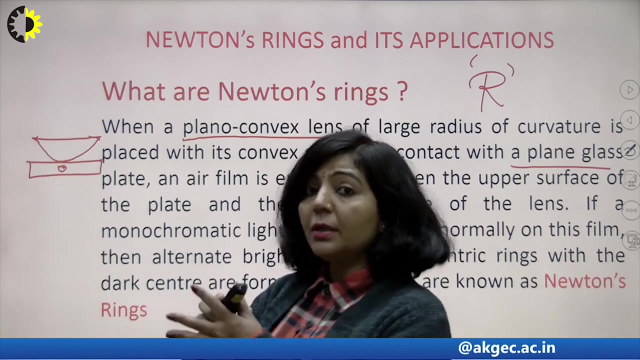 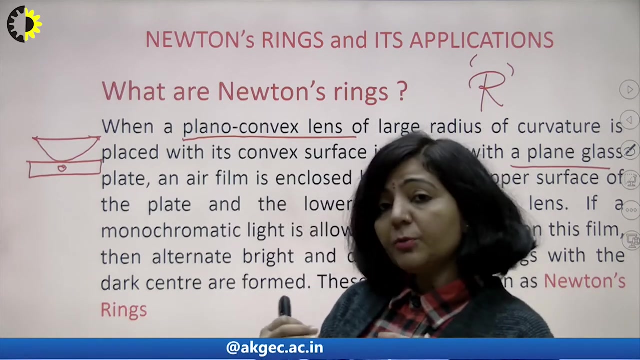 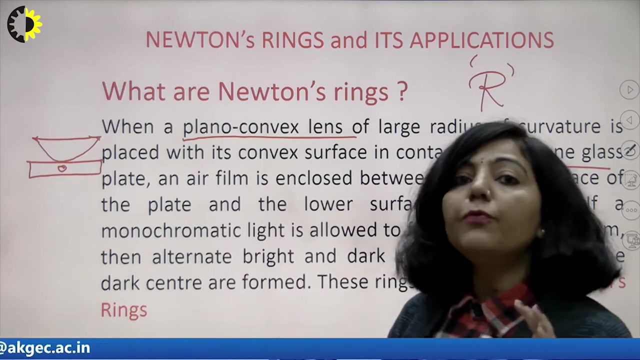 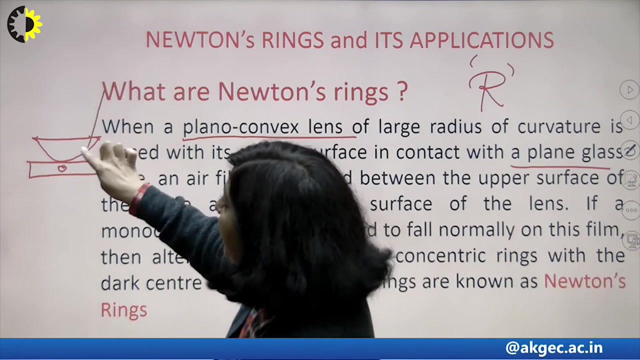 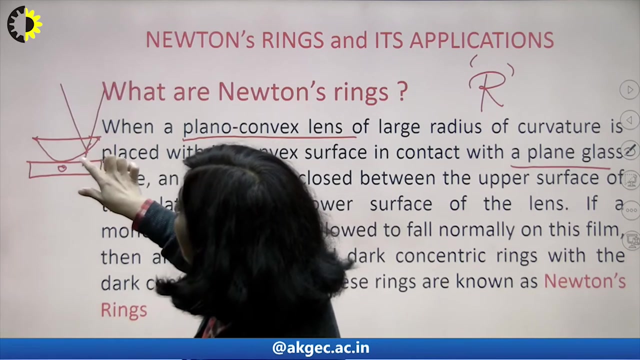 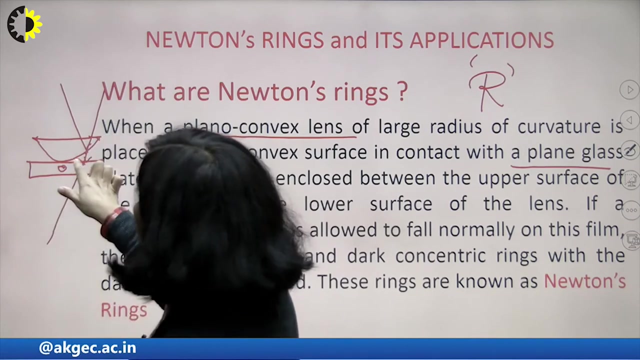 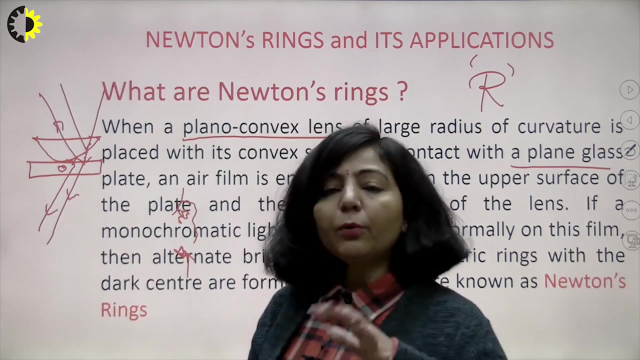 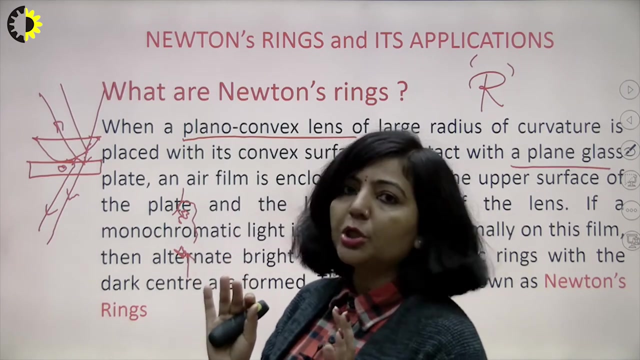 and how these rings are formed. So Newton ring experiment is a type of light ray that will go on dividing and since all these rays, they are coherent in nature, they are very close to each other, So they will get superimposed. and when these light rays will get superimposed you will get an interference. 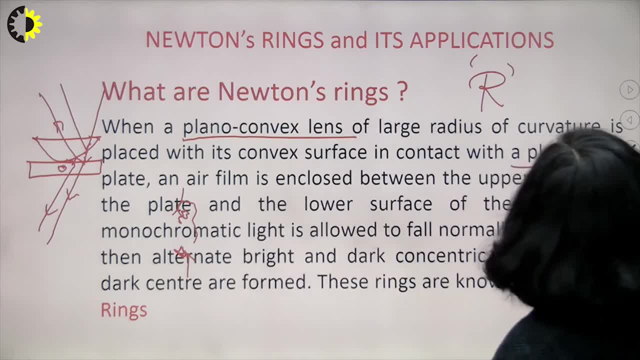 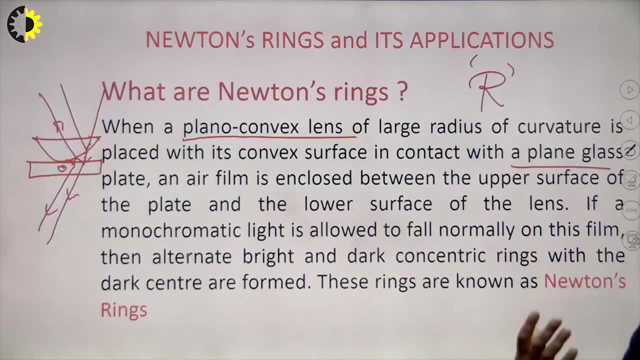 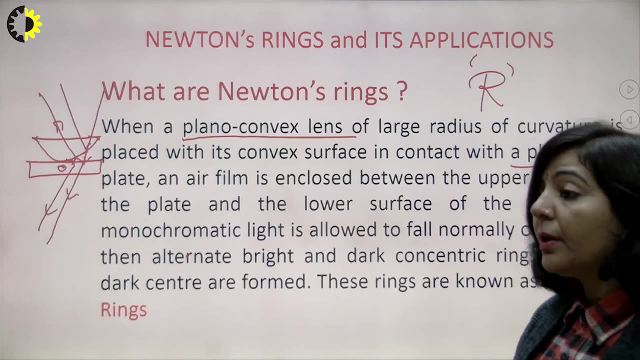 pattern and that interference pattern that will be in the form of concentric circles or rings. Why I am saying that you are going to get the interference pattern in the form of concentric circles or rings, or why only the rings, ring type of interference pattern is obtained. The reason is: since you are having this symmetrical, since you are having 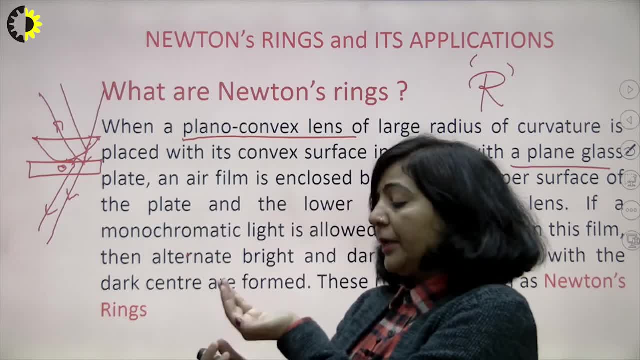 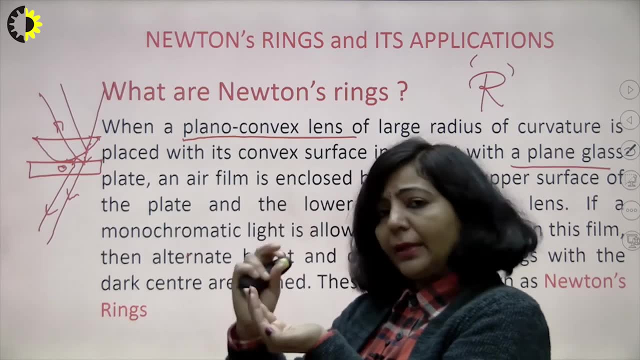 this curve part of plano, convex lens placed on glass plate, So you are having a symmetrical air film on all the sides of point of contact. So for a particular thickness, if you are taking thickness T, then for that particular thickness, if you will join all the points, 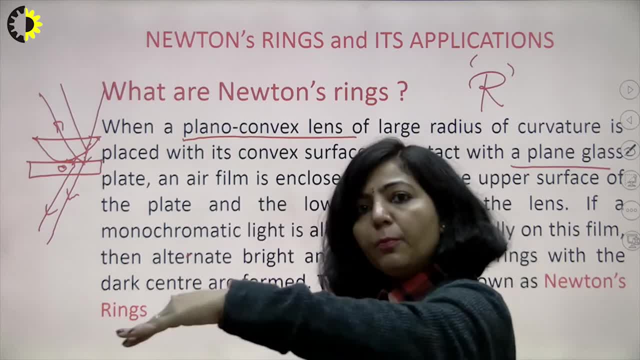 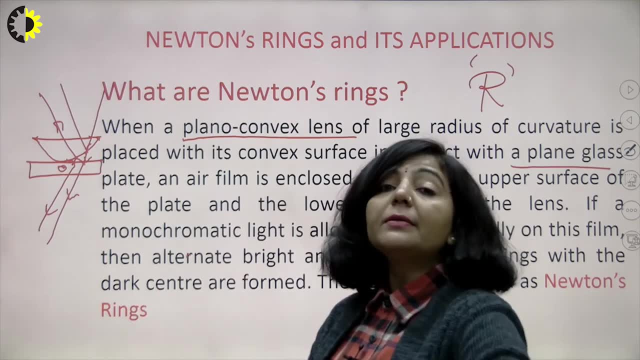 of same thickness, then that will form a circle. So over a certain point where you are having a constant thickness, then you are joining all those points, then it will form a circle. So that is the reason, since you are having a symmetrical air film on all the sides of 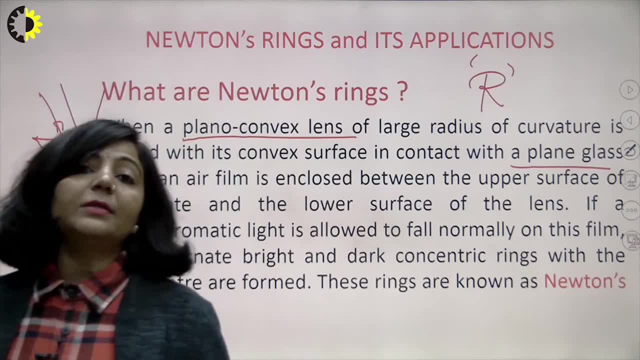 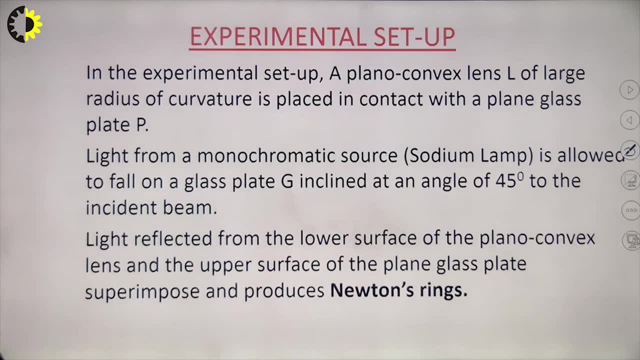 point of contact. So, because of this reason, we are getting this interference pattern in the form of concentric circles or rings. Next one is the experimental setup. So, as I have mentioned that, you have a plano convex lens and that plano convex lens is of large radius. 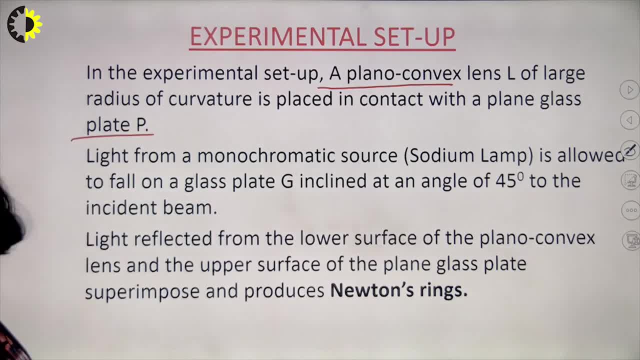 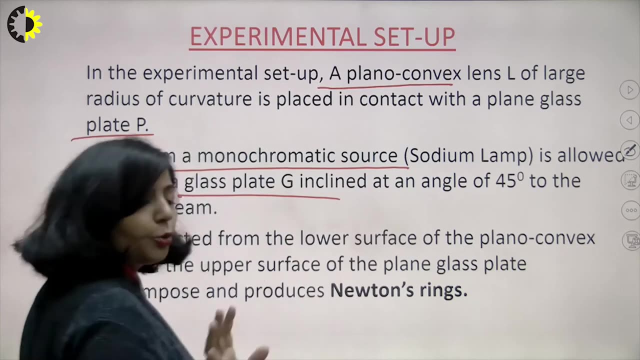 of curvature and it is placed upon a glass plate. There is a monochromatic source of light. suppose you have sodium, You know sodium lamp that gives us yellow light, that light of single wavelength. So you have a monochromatic source of light. after this, there is a glass plate. I will show you. 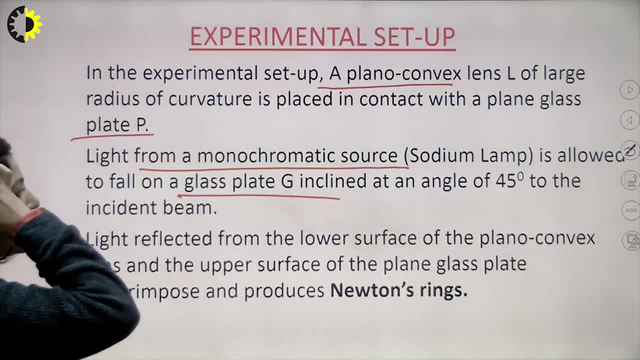 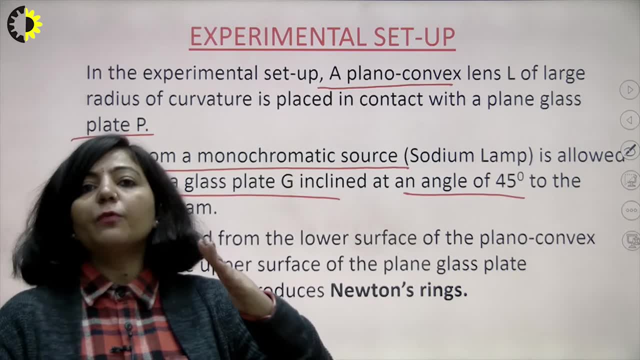 that experimental setup. but before that I am describing all these components here. So you have a glass plate and that glass plate is inclined at an angle of 45 degree to the direction of incidence of light. So suppose the light rays are coming along this direction. 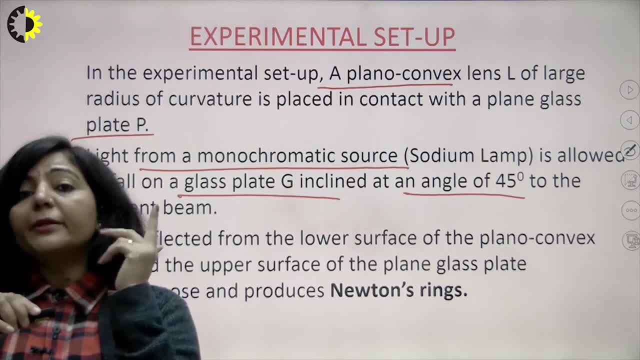 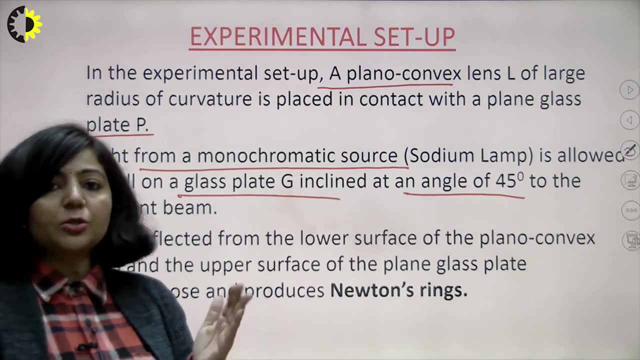 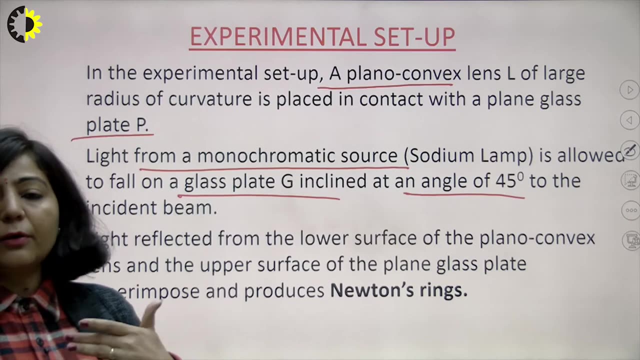 then the glass plate that makes an angle of 45 degree but the incidence of incidence with the those incident light rays. After this the light will incident over this combination, over the air film that will be between plano convex lens and glass plate and there over. 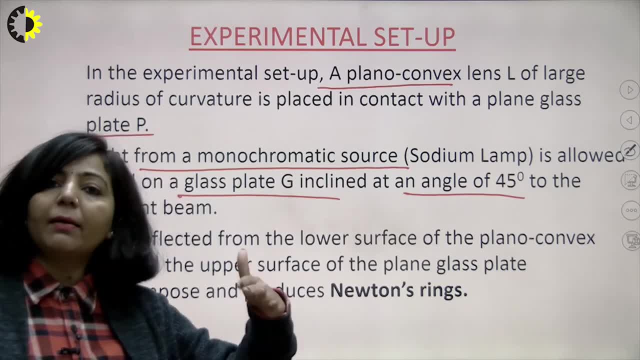 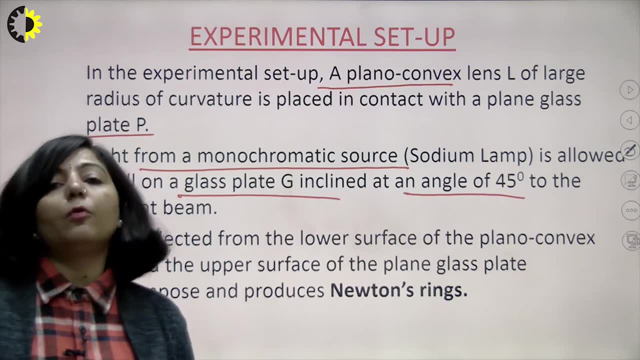 that air film there will be. division of amplitude means a single light ray, its amplitude will go on dividing and you will get large number of four coherent rays which will get superimposed and you will get an interference pattern. So now let me show you that experimental. 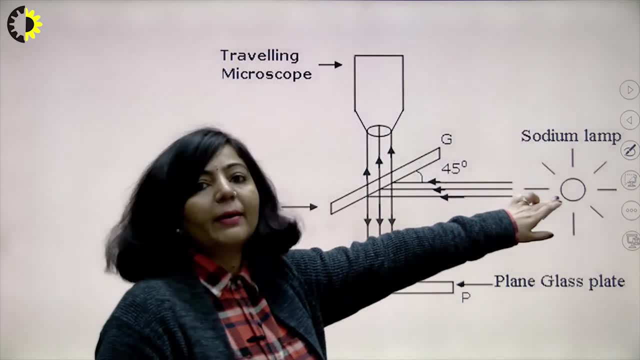 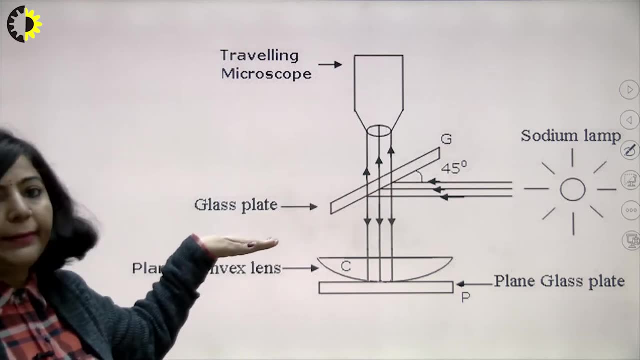 setup here. So, as you can see, this is the sodium lamp monochromatic source of light. this is your monochromatic source of light. this one is the glass plate which is inclined at 45 degree to the direction of incidence of light. it is making 45 degree angle here. 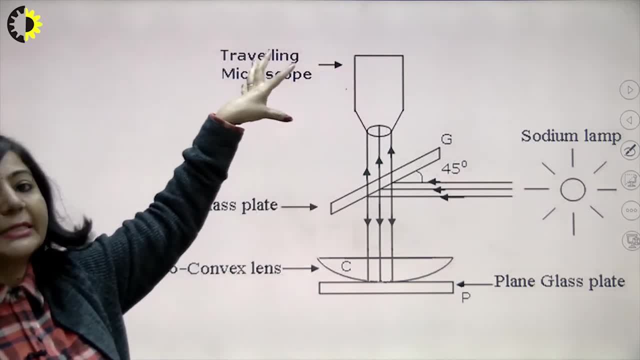 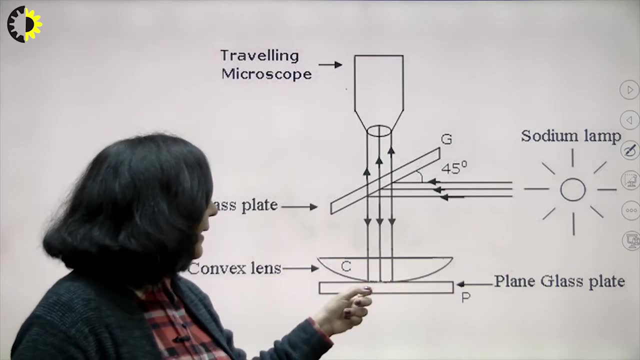 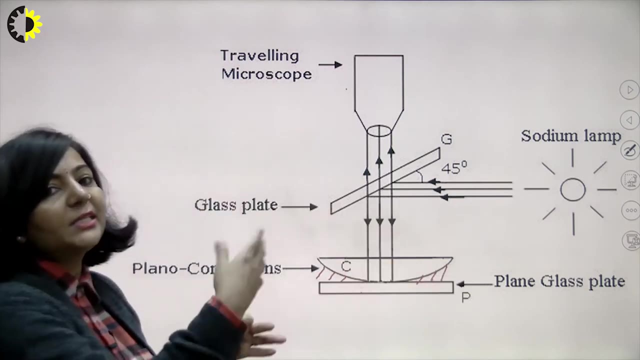 and this one is travelling microscope through which you will observe this entire interference pattern. So the position of observer is this one. you have this plano, convex lens and glass plate here. So in between this plano, convex lens and glass plate, you are having a symmetrical air film on all the sides. So this one is 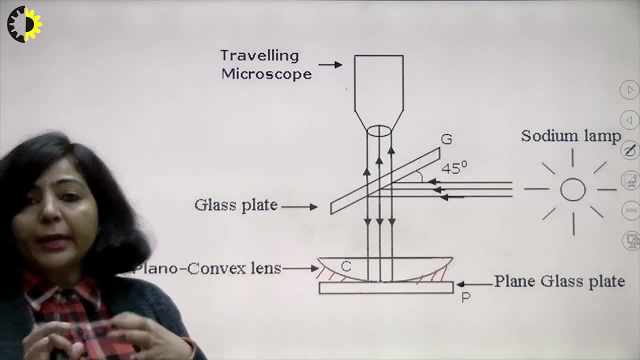 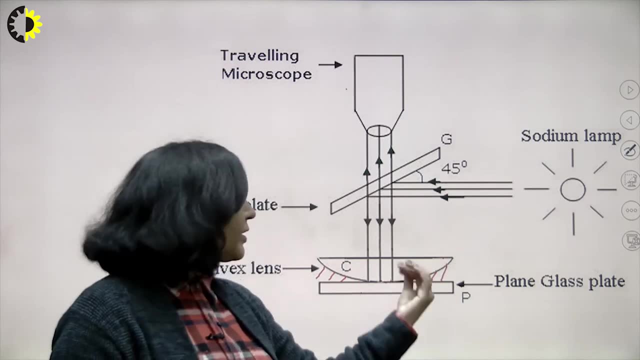 plano convex lens. this is glass plate and the interference pattern basically that will take. that will be observed through to due to multiple reflection and refraction of light rays from this air film. So the air film will be between- if I am saying this is x and 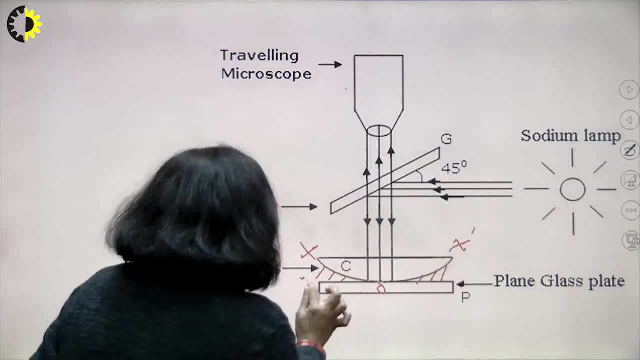 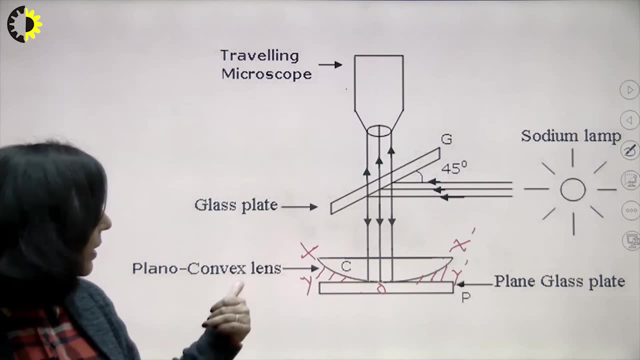 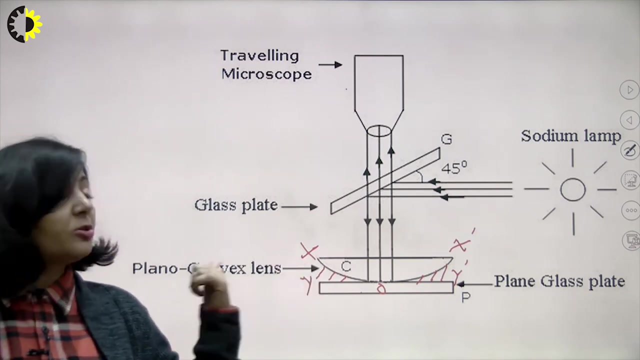 this is o, this is x dash, then this one is y o y dash. So what is x o x dash? basically, that represents the curve part of plano convex lens, and y o y dash that represents the upper part of that glass plate, So that air film is between these two and when the light will. 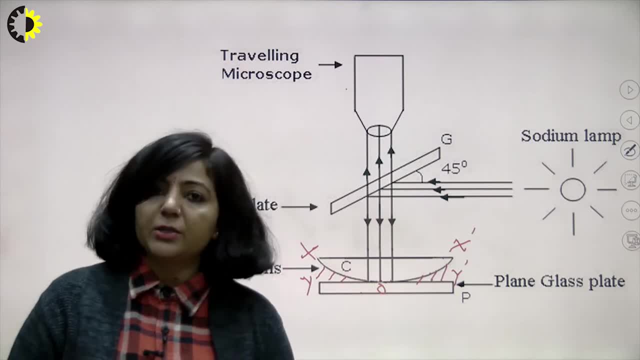 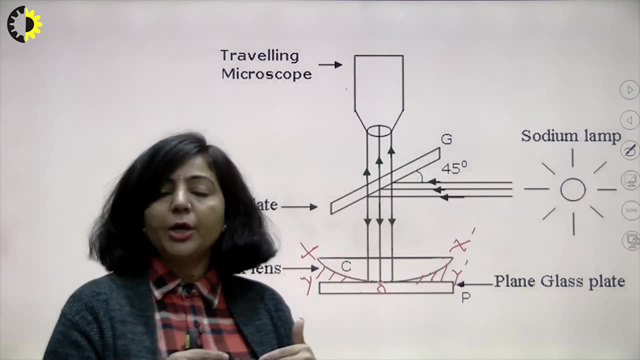 strike over the upper part of air. film means when light will strike over x o, x dash part. some part will be reflected, some will be transmitted. then light will reach over y o, y dash again. some part will be reflected, some will be refracted. again, the reflected part will reach over the. 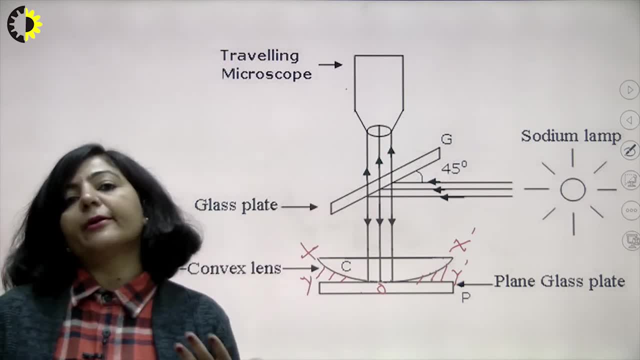 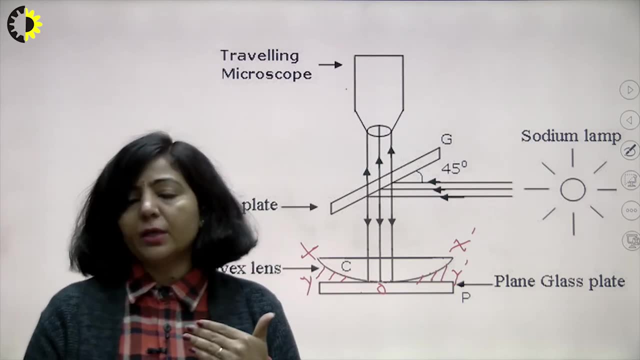 upper part of air film. some again, some part will be reflected, refracted, and this process will go on. you will get reflected rays which are very close to each other. you will get transmitted, or you can say refracted- rays which are very close to each other. they will 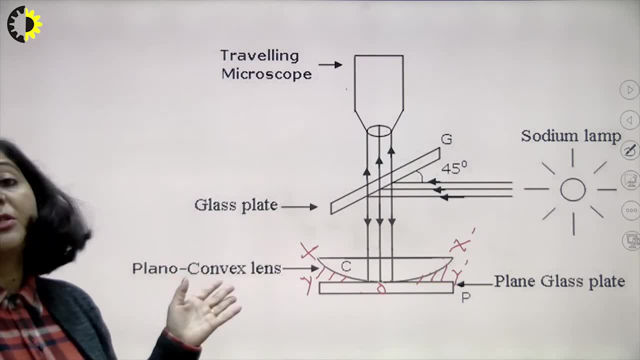 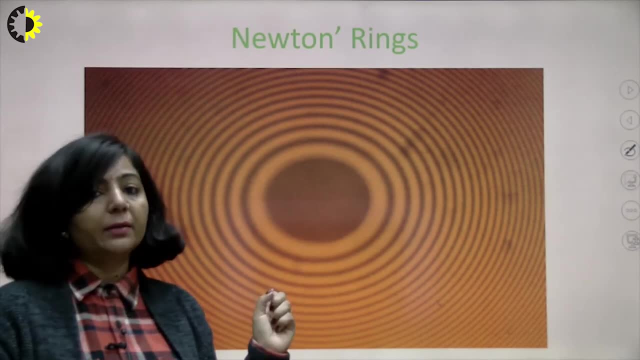 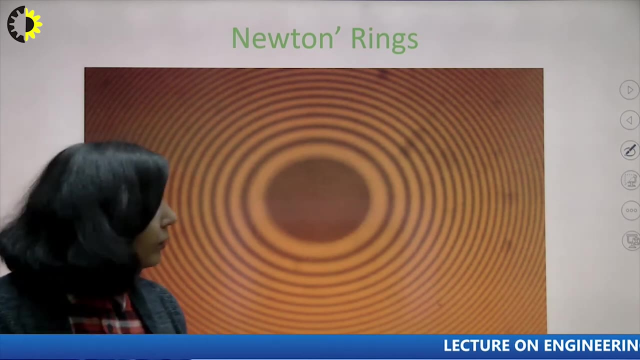 get superimposed and you will get an interference pattern. So this is the experimental setup of Newton ring experiment and this is the type of interference pattern. this is basically the interference pattern of Newton's ring experiment with the help of yellow light source. When you are using a yellow light source or a sodium lamp, then this type of interference 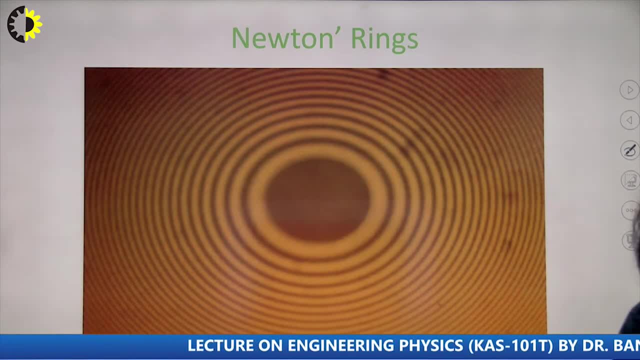 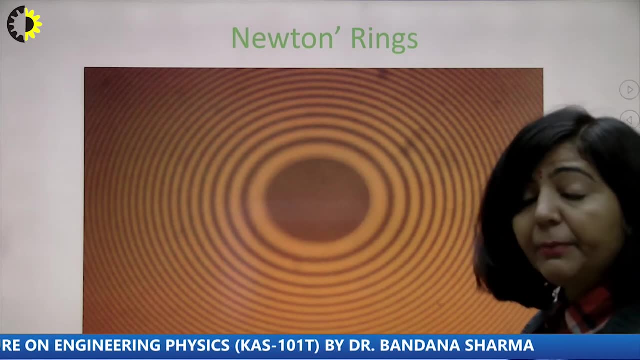 pattern is observed at the center. you are going to get a dark ring. then you are getting alternate maximas and minimas. So wherever the condition of maxima will get set will be satisfied. you are going to get maxima there and if the condition of minima is satisfied, 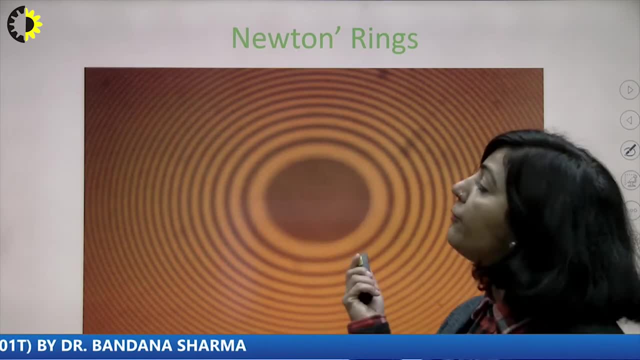 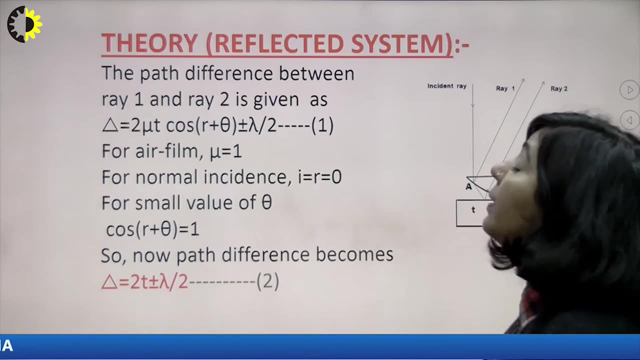 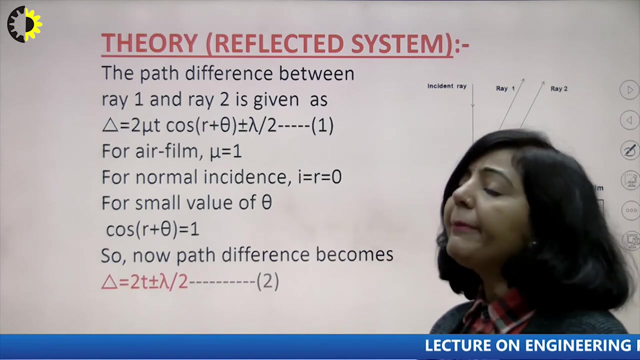 at over a certain point, then you will get minima. So this is the type of interference pattern which you are going to observe through Newton ring experiment, right. Next one is that in reflected system, what are the conditions of maximas and minimas and what will be the 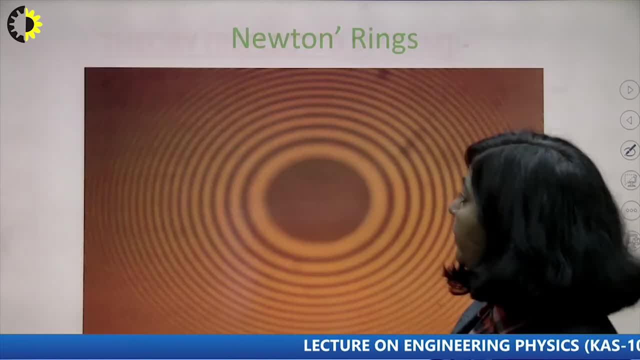 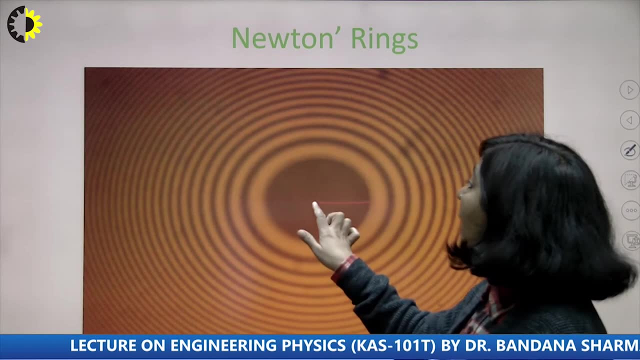 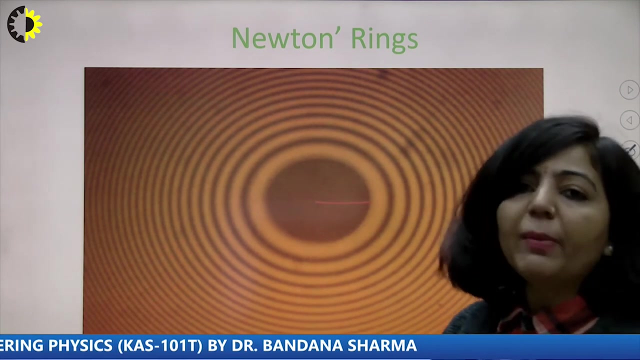 diameter of bright and dark rings means we are going to find the diameter of these bright rings. we will find the diameter of these dark rings which will be observed in this interference pattern So easily using the property of circle, using simple geometry, we can find that diameter of bright and dark rings. So let us calculate. 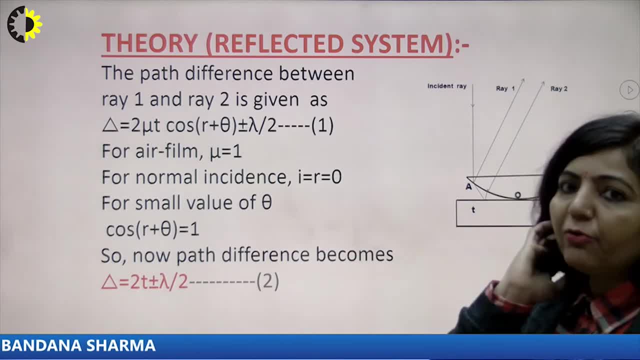 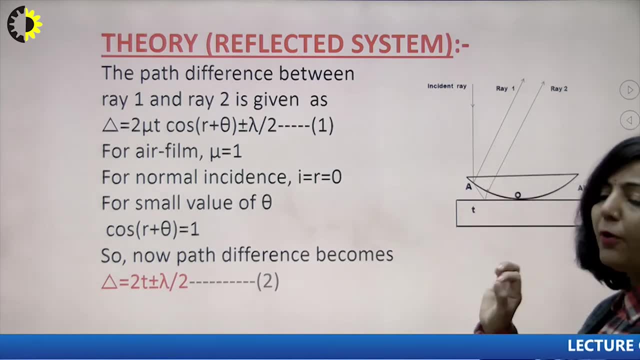 that diameter of bright and dark rings here. So we are going to start with the reflected system. as you know, this is a bed shade film. you are having this thin film of non-uniform thickness between this plano, convex lens and glass plate. You can see here this particular 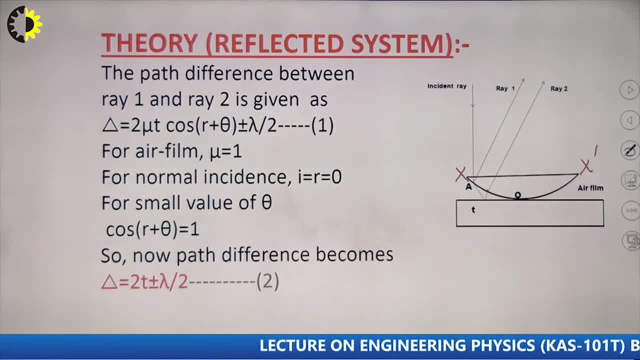 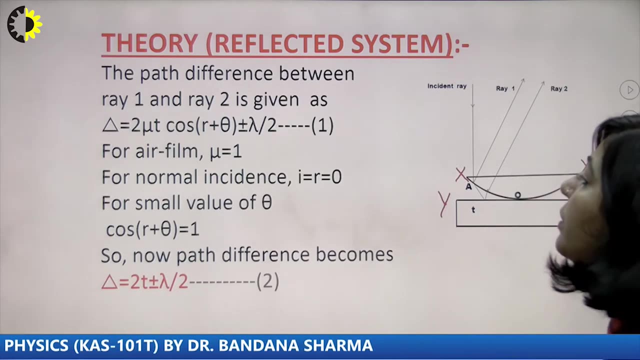 part. xox dash is the upper part of this air film and yoy dash, that represents the lower part of this air film, and that air film is between xox dash and yoy dash. So, since it is a bed shade film and we all know the results of a bed shade film, So 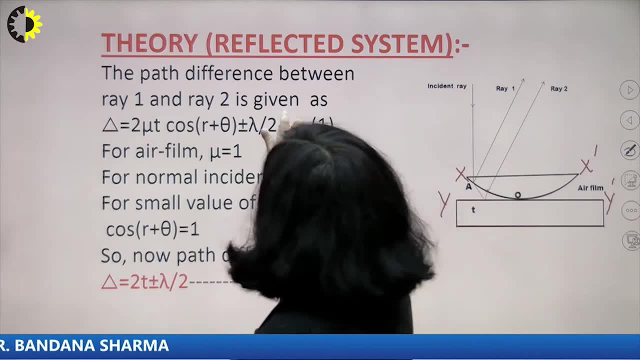 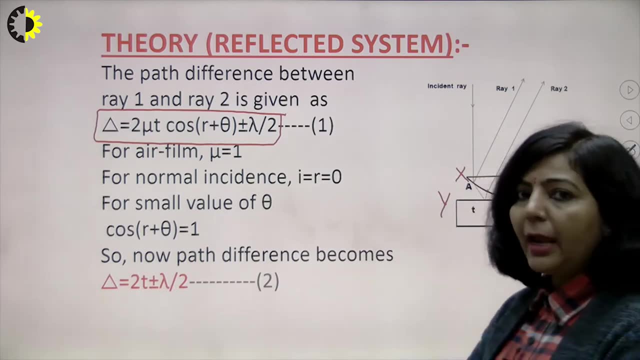 in reflected system, since the part difference between the reflected rays, that is equal to 2, mu, t, cos, r plus theta plus minus lambda by 2, that we have already calculated in our last lecture of bed shade film. So the part difference for a bed shade film in reflected 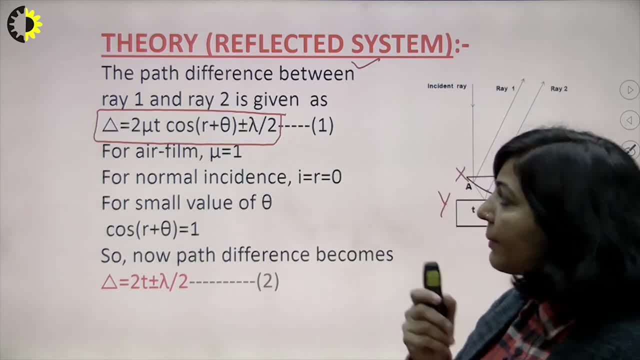 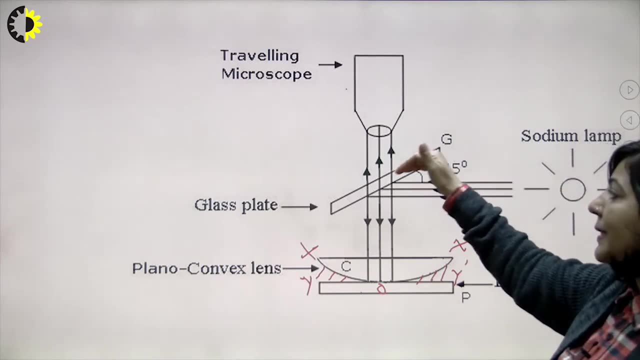 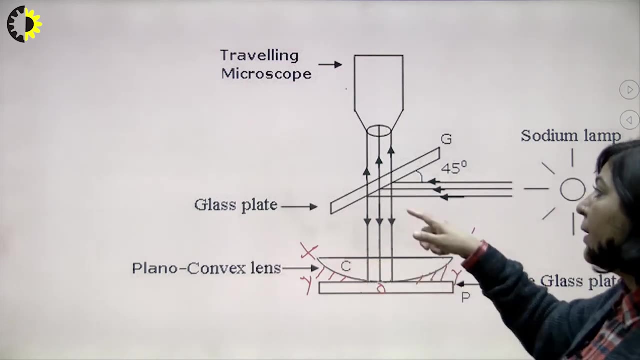 system is 2 mu, t, cos, r plus theta plus minus lambda by 2. here Now, as you can see in this experimental setup that when light will strike over this glass plate which is inclined at 45 degree, then the reflected rays, they will move towards this air film, So light will. 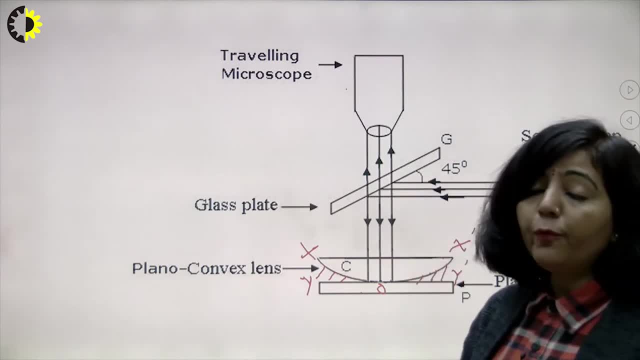 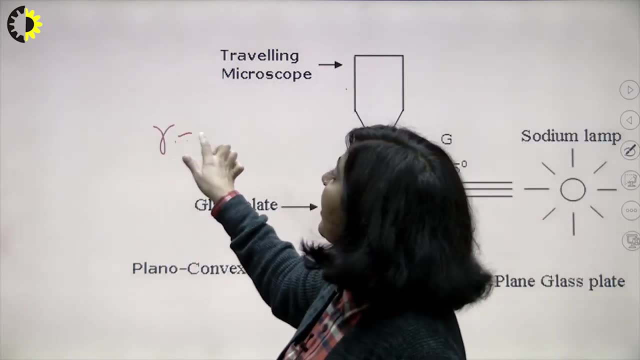 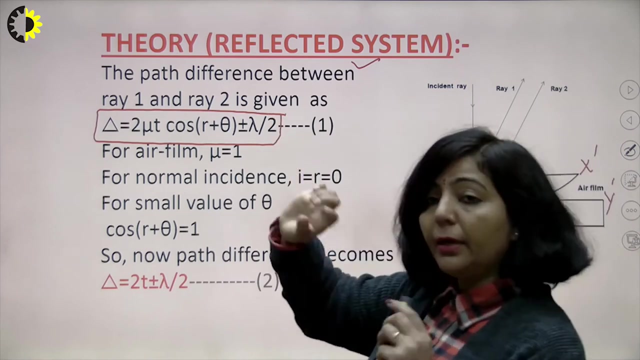 incident normally here. So there will be normal incidence of light in this arrangement of Newton ring experiment. So you know when light will incident normally, then angle of refraction will be 0.. So that is a reason I am going to write here that for this air. 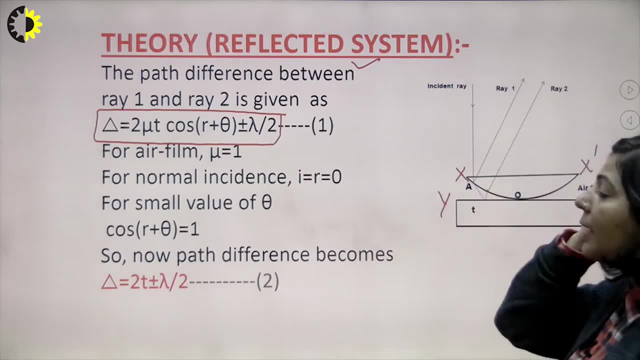 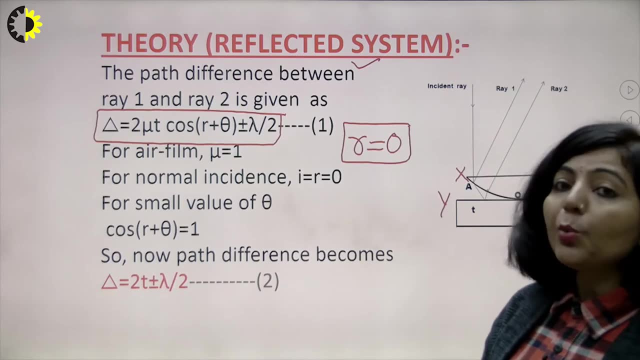 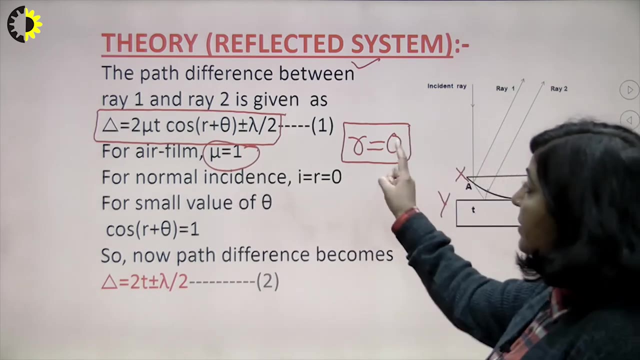 film which is In between planar convex lens and glass plate. since light will incident, normally, So r is equal to 0 and r 0, and since you are having an air film, So you know for air the reflective index is equal to 1.. So r 0 and mu 1 and cos r plus theta, that will be equal to cos. 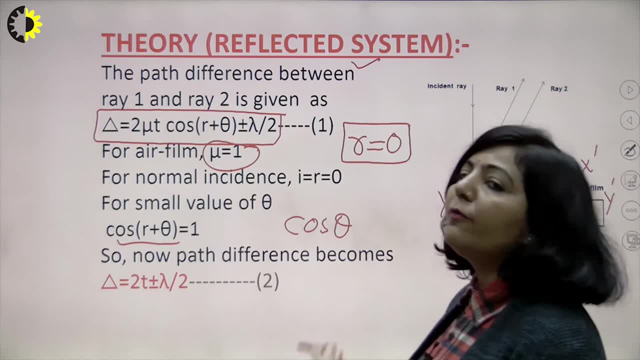 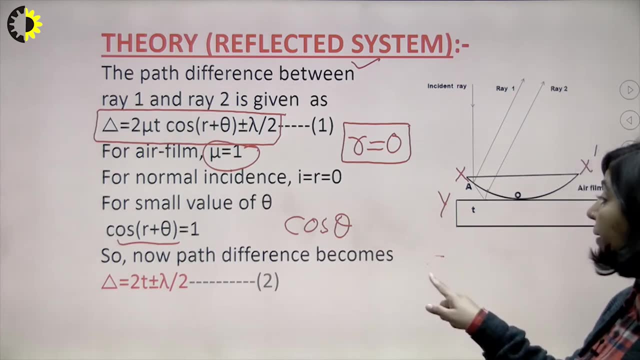 theta, because r is already 0 and you know, for small value of theta, since theta is very small, that angle between x o x dash and y o y dash is very small. So because of that reason, this for small value of theta, cos theta is approximately: 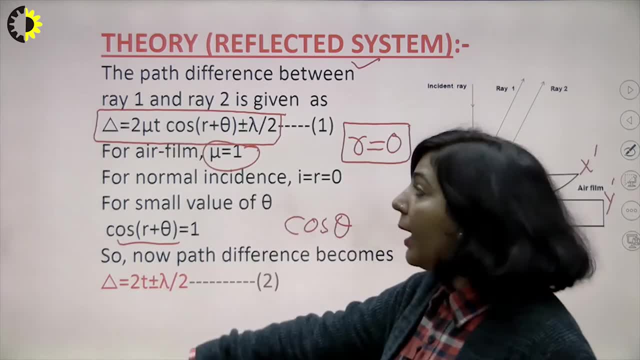 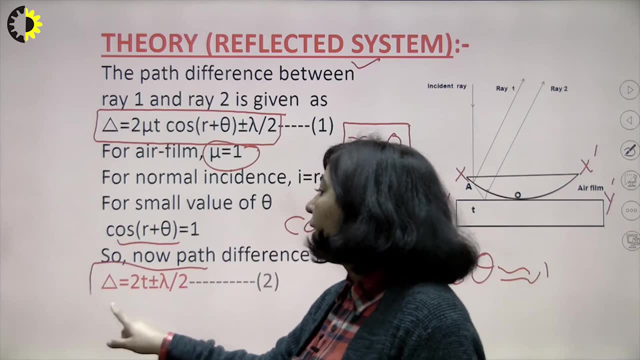 1. It means this particular part is going to give you 1 and since you are having that air film in between planar convex lens and glass plate, So you are getting delta as 2 t plus minus lambda by 2.. So I hope the meaning of this one is clear, Since you are 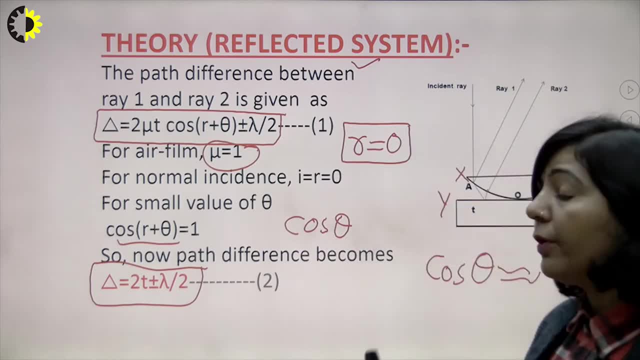 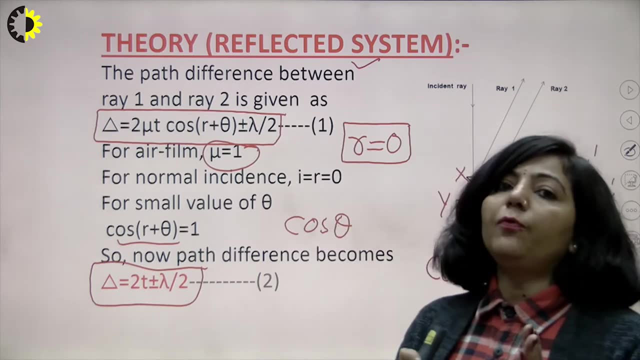 having an air film between planar convex lens and glass plate for air reflective index is 1.. Since the light is incident, light will incident normally over that area. So you know that arrangement of air film between planar convex lens and glass plate, That is. 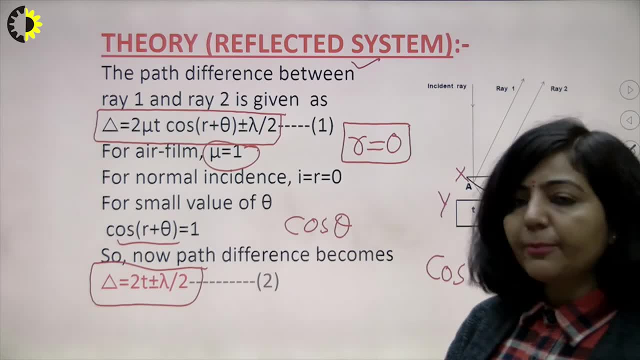 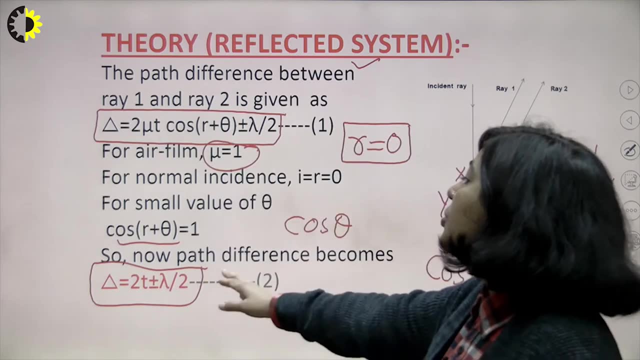 why r is 0 and for small value of theta. cos theta is approximately 1.. That is a reason. this entire factor is going to give you 1 and this mu is. this mu is also going to give you 1.. So this equation number 2, that represents the effective part difference here. So now, 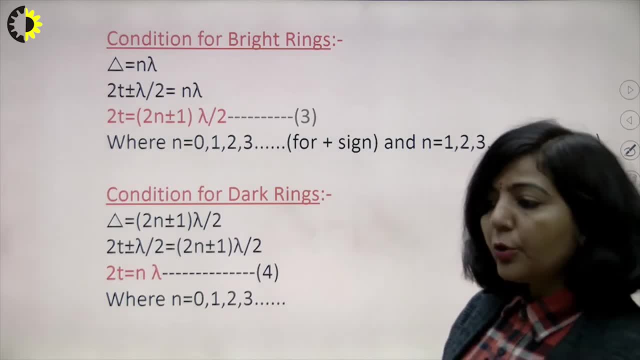 we are going to find the diameter of bright rings. So if I am saying bright ring, it means over those points. 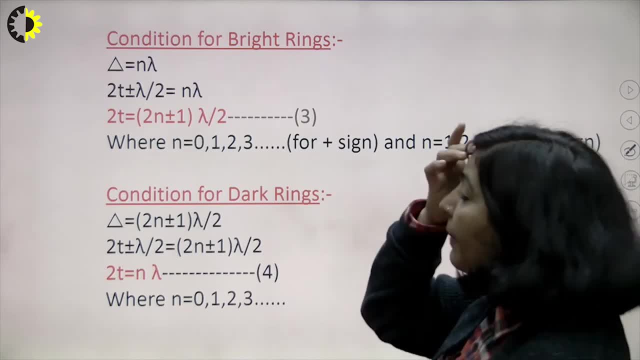 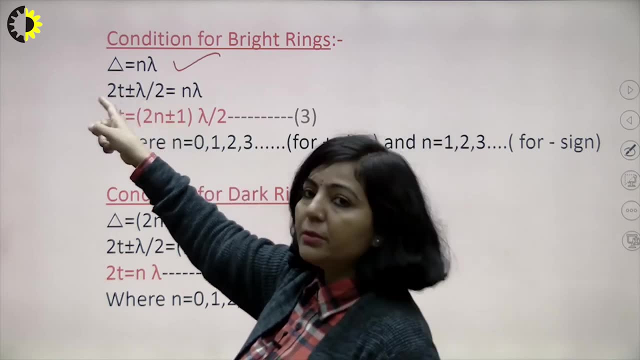 the condition of maxima will get, will be satisfied. so for maxima, you know the power difference should be l lambda, or you can say even multiple of lambda by 2. and you know the power difference in newton ring experiment it is 2t plus minus lambda by 2. so substitute this delta here and 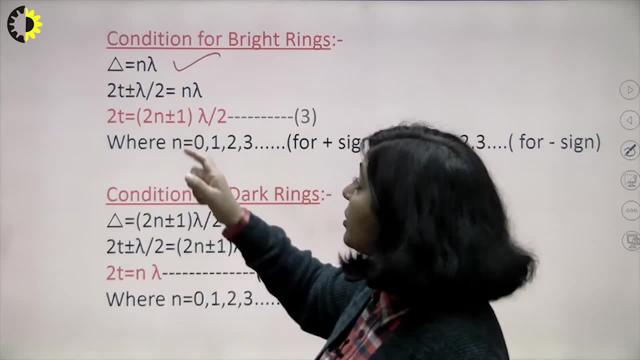 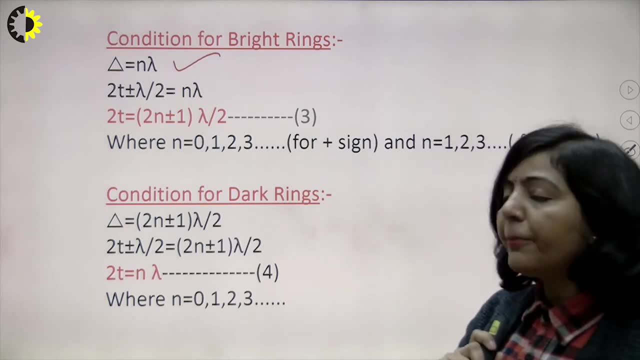 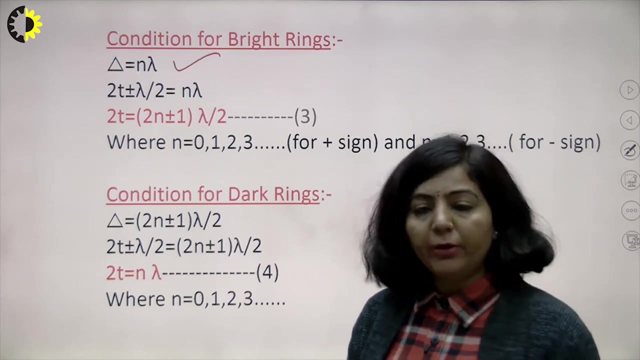 that is equal to l lambda. now simplify it. after simplifying you are getting. the condition is: 2t is equal to 2n plus minus 1 lambda by 2. this is the condition for bright ring and using this condition we will find the diameter of those bright rings and similarly, you can decide the. 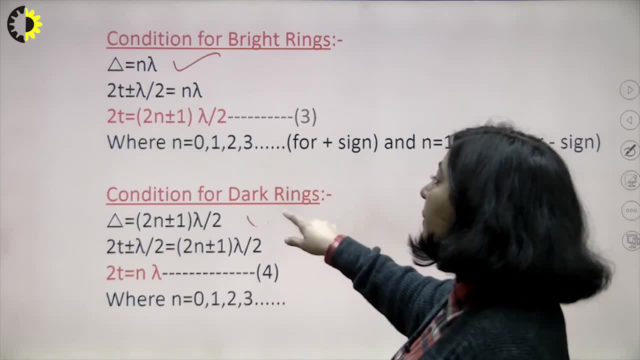 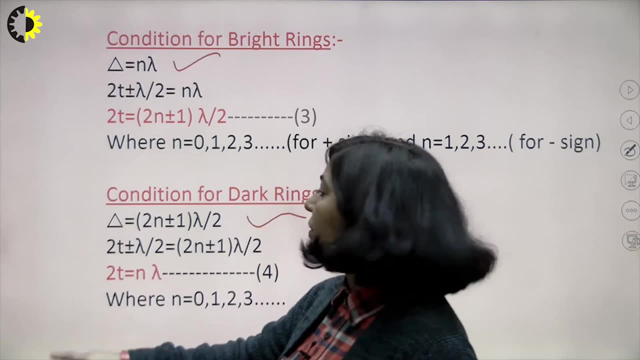 condition of minima and the condition of minima is for minima. the power difference should be odd multiple of lambda by 2. so this is the expression and you know what is the power difference for newton ring experiment. it is simply 2t plus minus lambda by 2. so after substitution and simplifying, 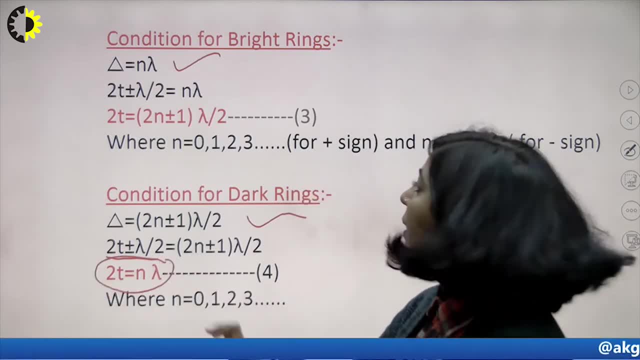 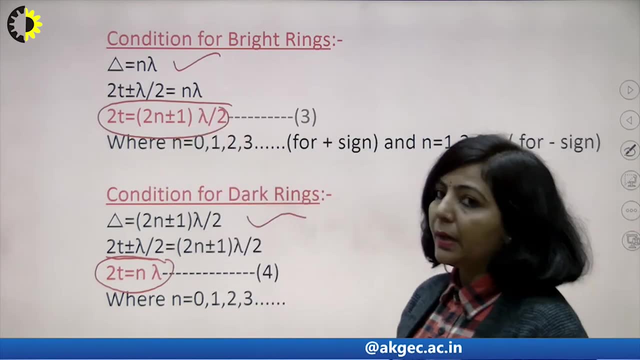 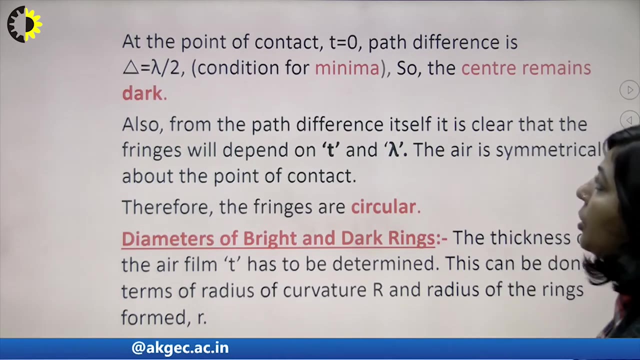 you are getting that equation number 4 is for minima and equation number 3 is for maxima. so 3: 3- this is for bright ring and the equation number 4 is for dark ring. so using these two conditions now we are going to find the diameter of bright and dark rings. so now i am starting with the 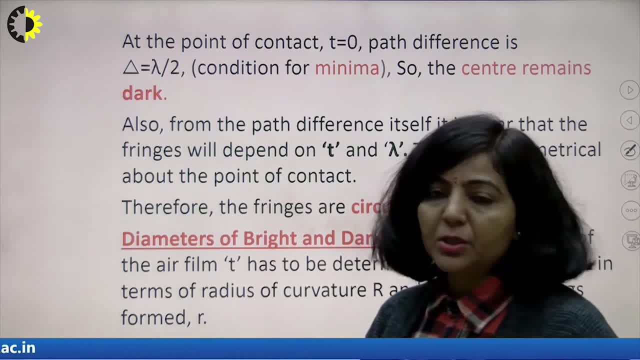 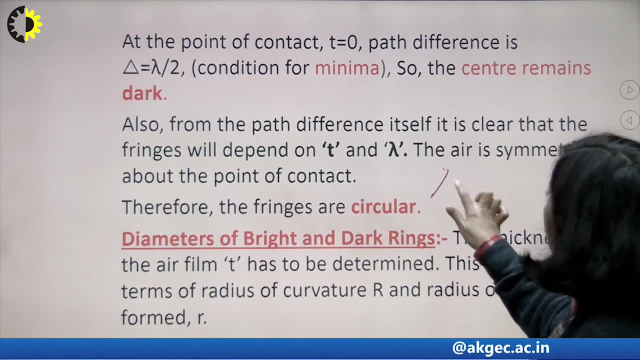 bright rings and the reason of this fact, fact that we are getting that interference pattern in the form of concentric circles or rings. the reason is very simple. this part difference. in case of newton ring experiment, it is simply 2t plus minus lambda by 2, so this is the difference. 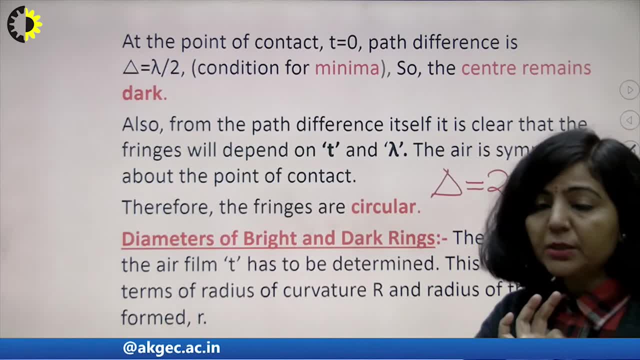 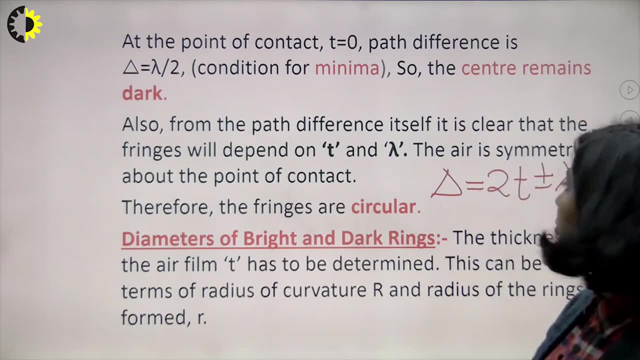 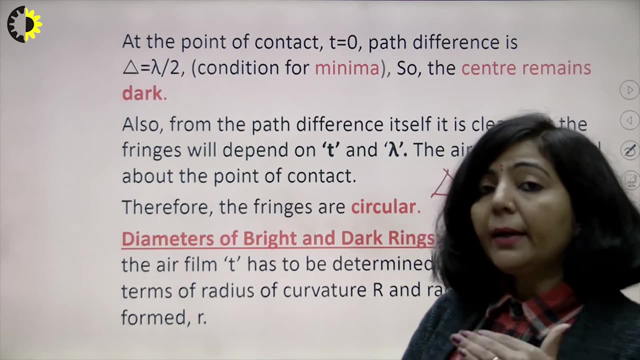 and, as you can see here, the first point is that in reflected system, at the centre, we are going to get a dark ring or a minima. what is the reason of this? if i am saying center, center means where the planar convex lens and glass plate, both are coinciding at that point of consisting. 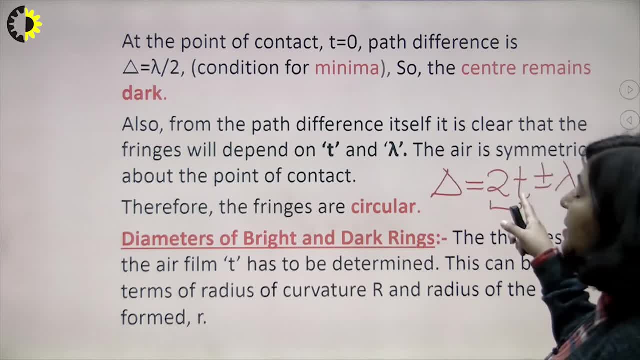 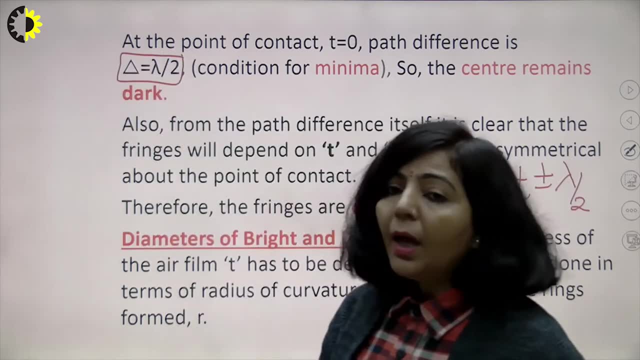 where those two are coinciding with each other. this t is 0, thickness is 0, and if i am saying thickness is 0, then what will be delta? delta will be simply lambda by 2, and you need to know that lambda by 2, and you know, odd multiple of lambda by 2, is the condition of minima. it means at the 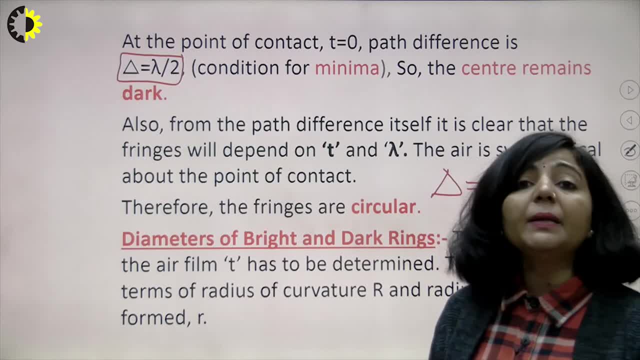 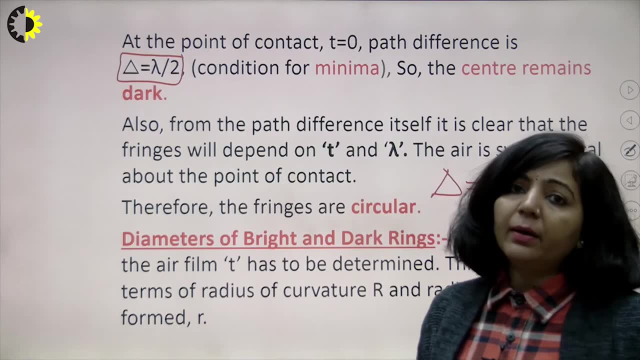 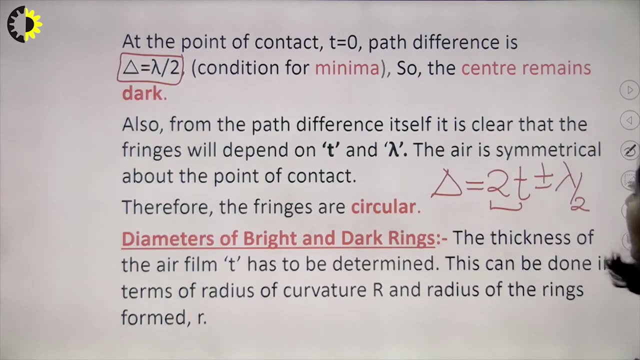 center in reflective system, the condition of minima will be satisfied, so that center will be dark. so alternate you will, then you will get bright, dark. bright dark means alternate. maximas and minimas are observed, but the center is dark. here and since the part difference itself gives, 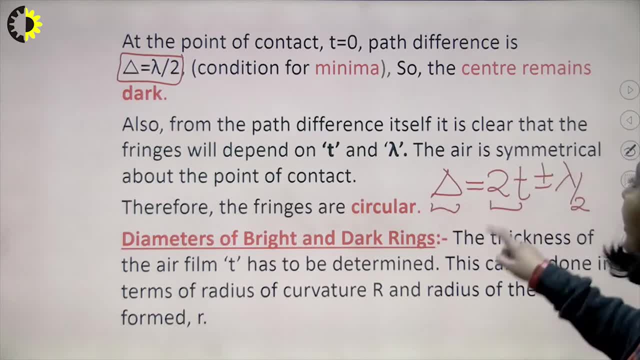 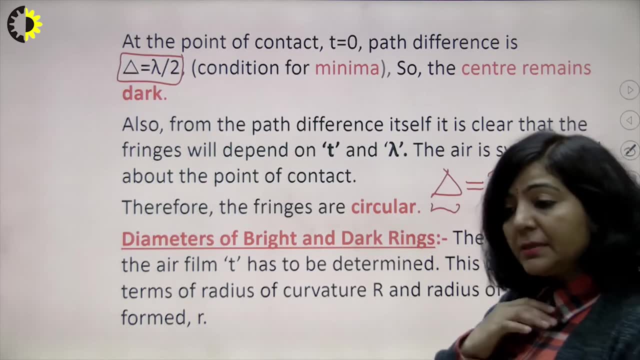 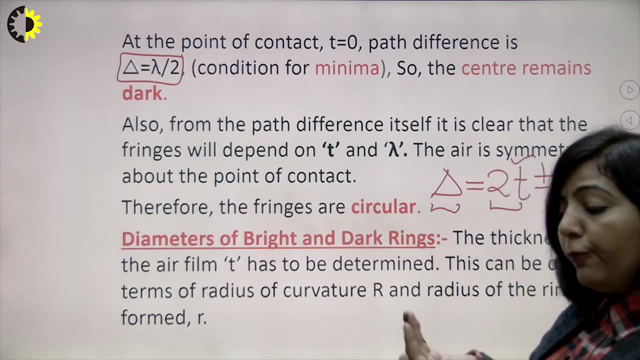 the condition since this part difference that depends upon the value of t and lambda and you know, if you are taking a monochromatic source of light then this lambda is constant. it means this delta is depending upon, depending only upon one factor, that is, thickness of that air film. so if 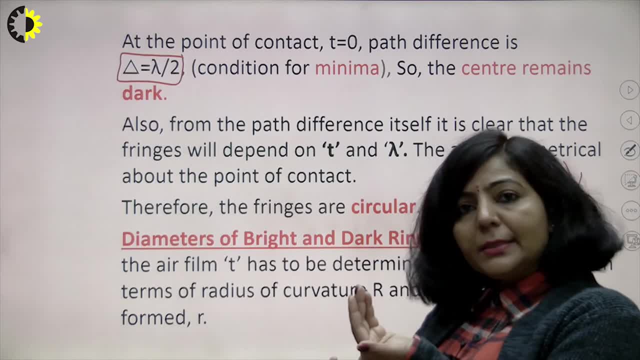 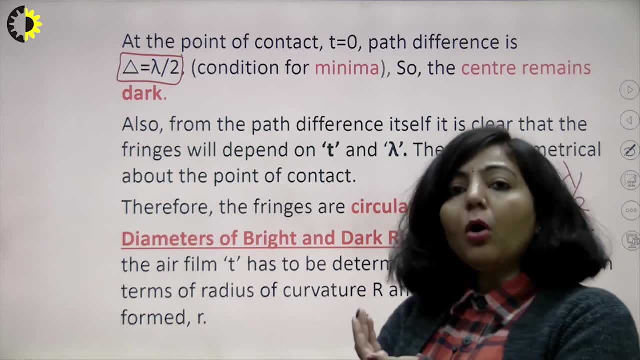 you are moving away from this point of contact, then at a certain distance the thickness of air film on all the sides of that point of contact will be same. so if you are joining all those points which are having same thickness, then that will form a circle. that is the reason you are getting concentric circles or rings. 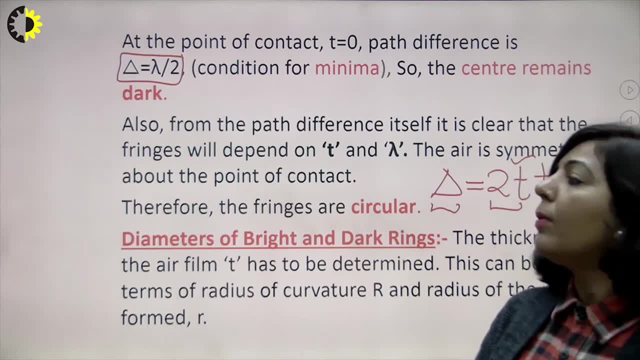 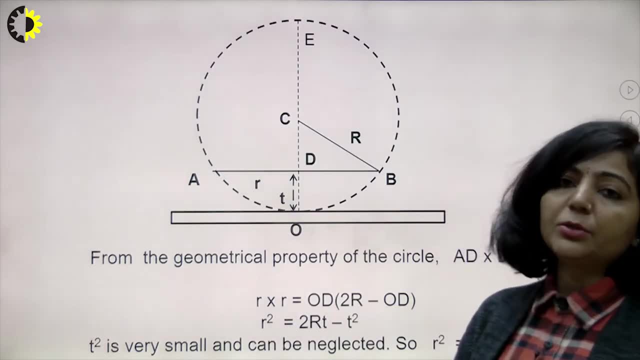 in this experiment, or the interference pattern is in the form of concentric circles or rings. so now we will calculate the diameter of bright and dark rings. so, in order to calculate the diameter of bright and dark rings, we are going to use the property of circle for this, again, you can. 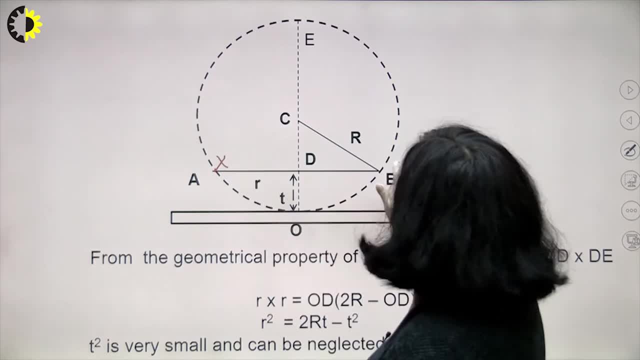 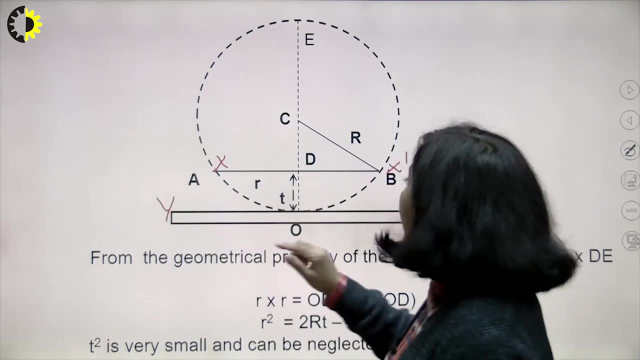 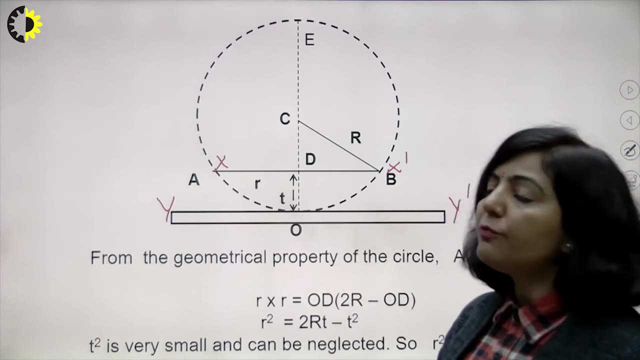 see here. this is your x o x dash means this is the curved part of that plano convex lens and this y o y dash, that is the upper part of your glass plate and the air film that is enclosed between x o x dash and y o y dash. now, in order to find the diameter of bright or dark rings, what we have done, 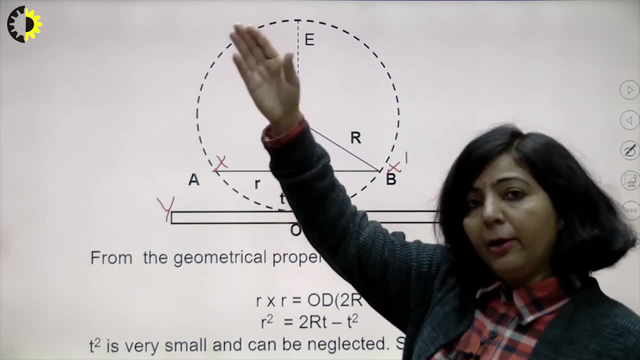 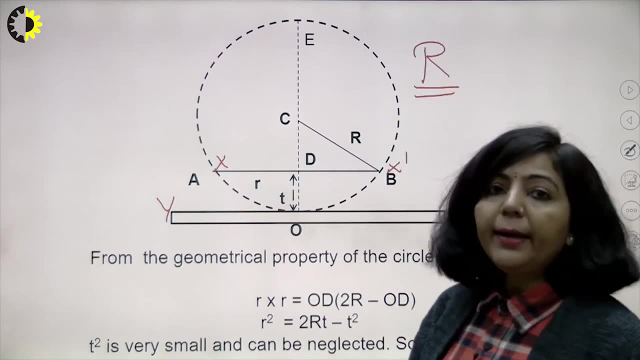 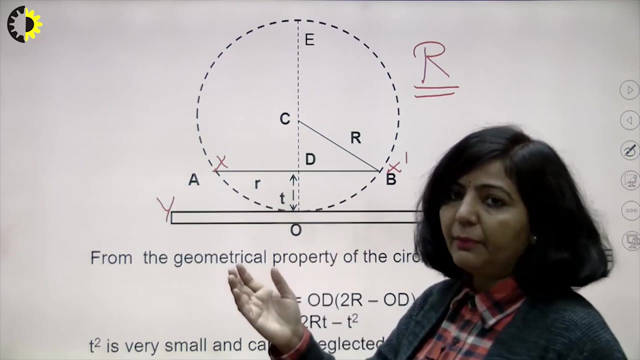 we have completed this uh curve part of that plano convex lens and, as i mentioned, that this plano convex lens is having a large radius of curvature, let that capital r is the radius of curvature. so if r is the radius of curvature, then this cb, which that will be equal to capital r, this ce. if this point is e, then ce is also r, this c. 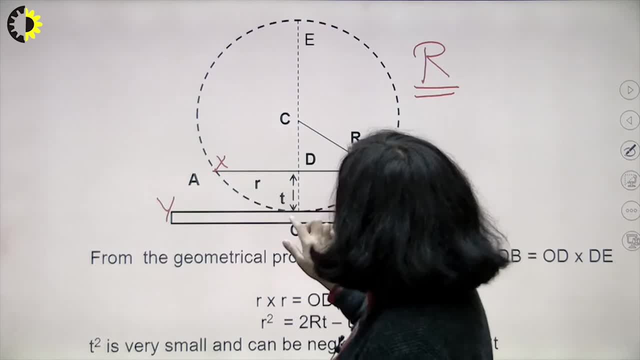 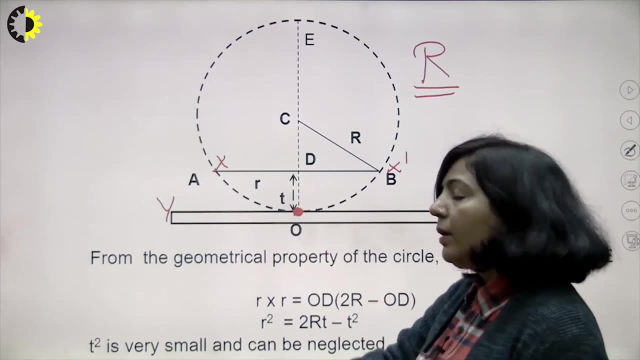 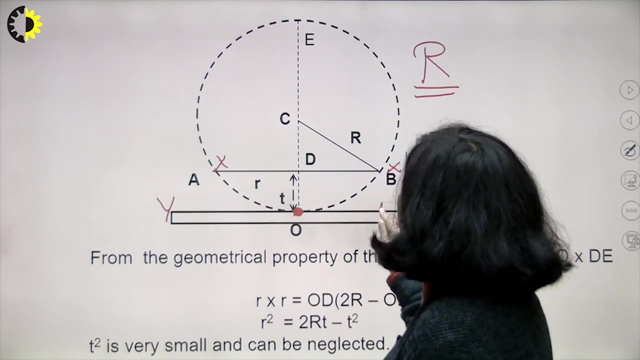 let this point is, let this point is o, then the ceo is also r. now, from this point o, which is the point of contact, suppose from this particular point of contact, at this particular distance, suppose at this distance, we are getting our nth maxima. if you are getting nth, 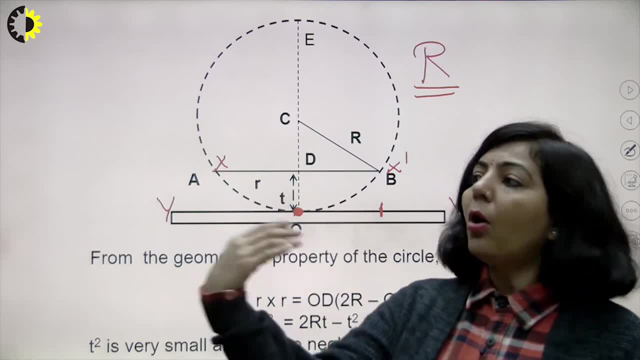 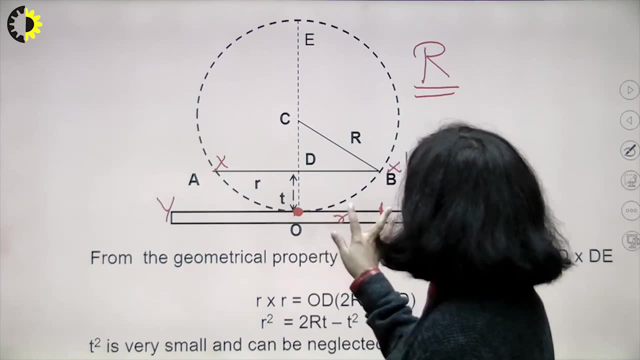 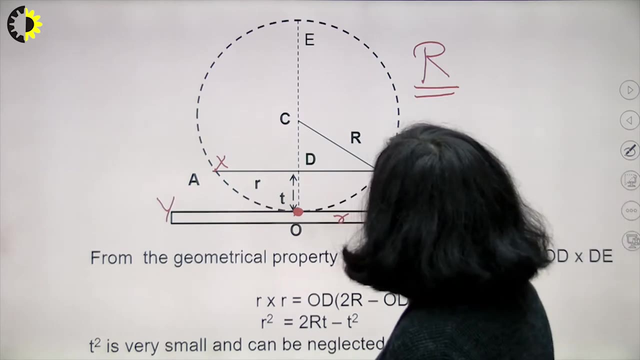 nth maxima. at this position, then, on all the sides, at same distance, we are going to get our nth maxima. so let this. this is r. this distance is r means it is representing radius of nth maxima. and what will be this? this will be thickness of your air film for nth maxima. 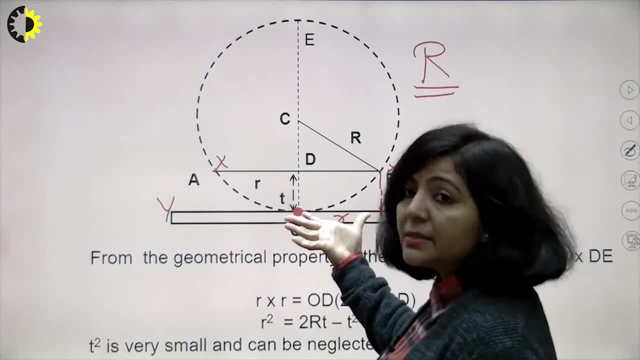 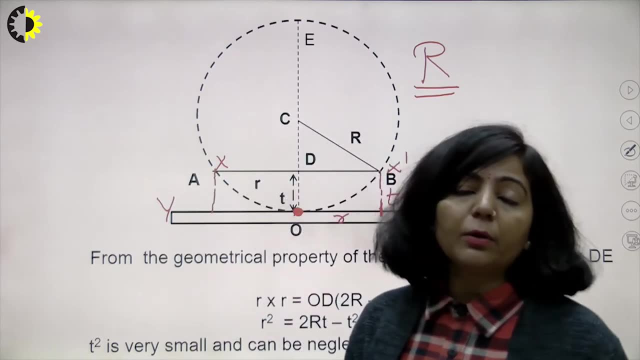 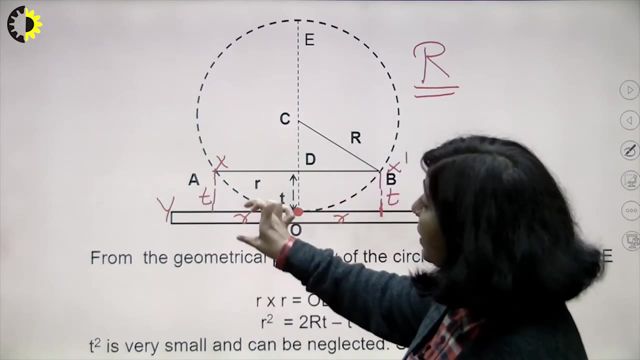 so if you are getting this, this, this distance as a radius of nth maxima along this direction, then on the other side, at the same distance you are going to get, you are going to observe your nth maxima. so this is again r, so this is r, this one is t. so if I am saying this, 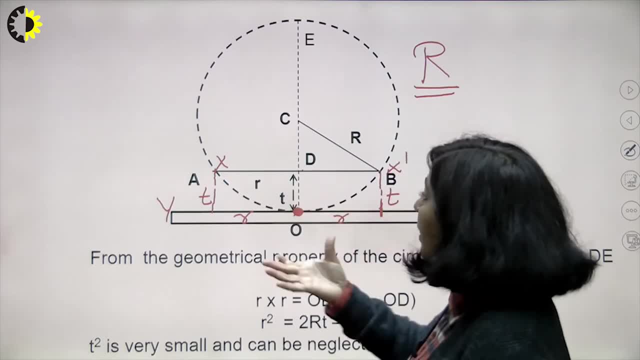 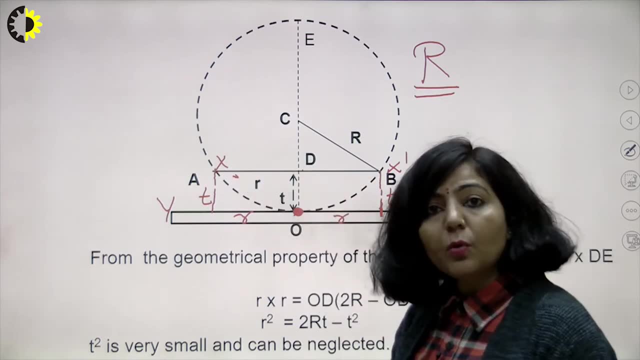 is t, then this part is also t, this part is also t. if this is r, then you know this particular part is also r. and if this is r, then you know this particular part is also r. now we are going to use geometry, we are going to use the property of circle and according to that, 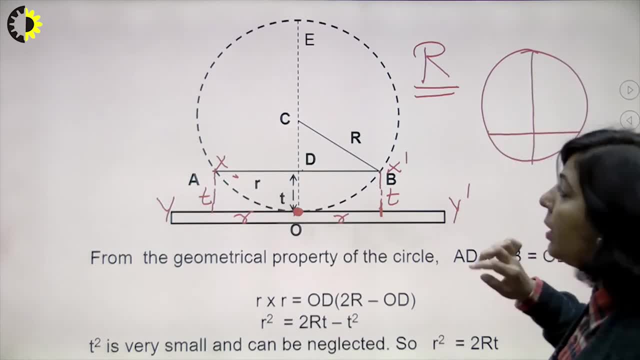 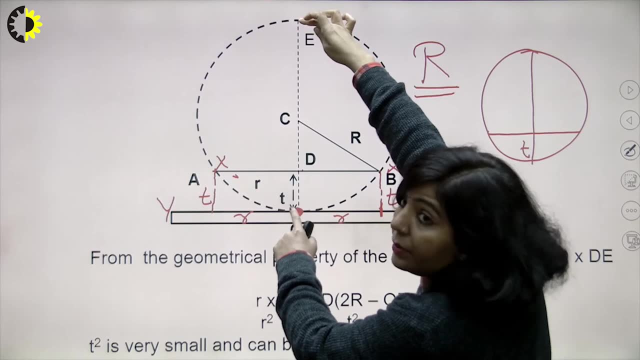 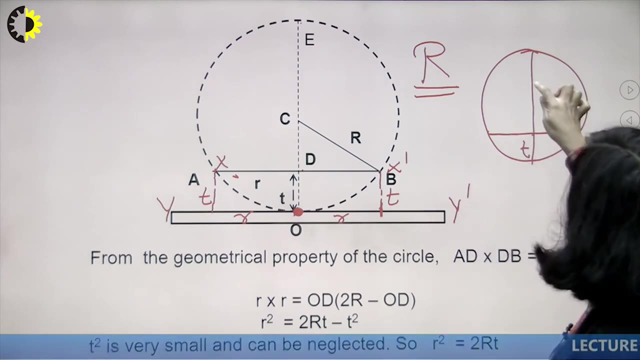 property of circle. if you are having these lines like this, you know this distance is T and this one is R. this is all. our total is. total is 2 R. so total is 2 R. and if you are subtracting this part T from this, then it will be 2 R minus T, so this particular portion is 2 R minus T. 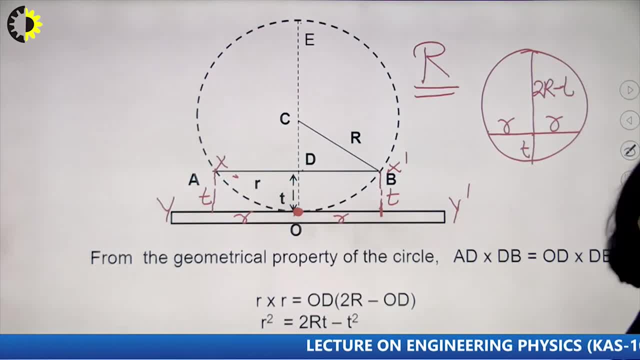 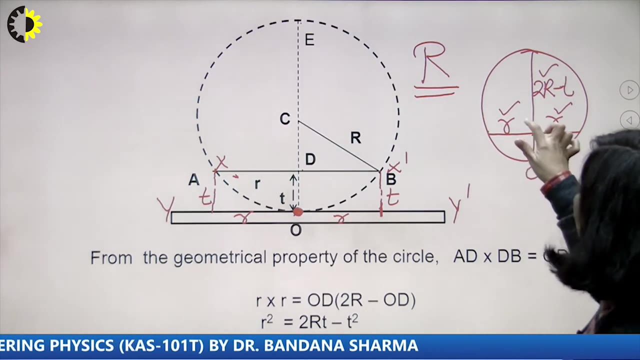 this is T, this is your R, this is R. so, according to the property of circle, the product of this and this part means product of R and R that will be equal to product of this part and this part. so, using the same property, what you have here, this point is O, this one is D, this point is your E and this point is let. 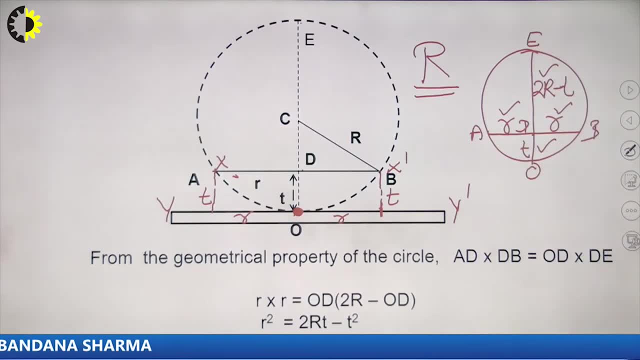 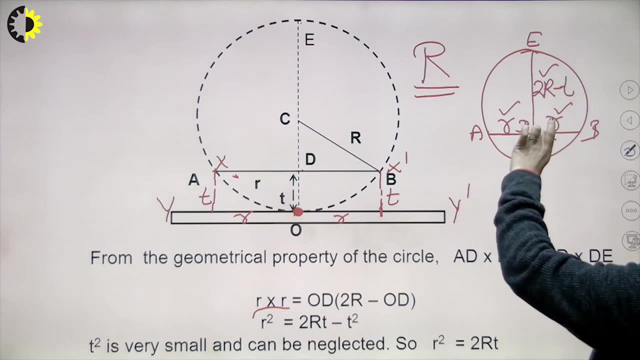 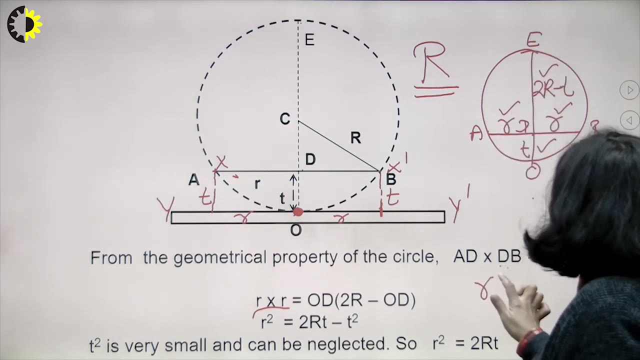 this point is a and this one is B. so according to down property of circle, this x. this means R into R. so this R into R is equal to this particular portion OD, which is T. so T alkaline into this portion, that is 2r minus t. so we have r square into 2r minus t into t. so what you are. 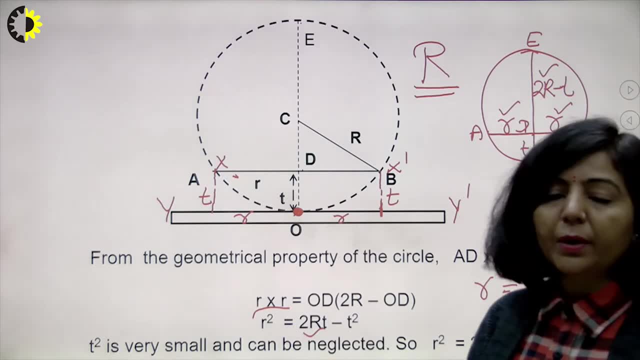 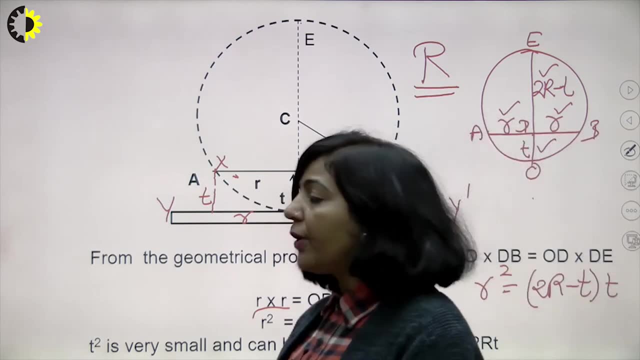 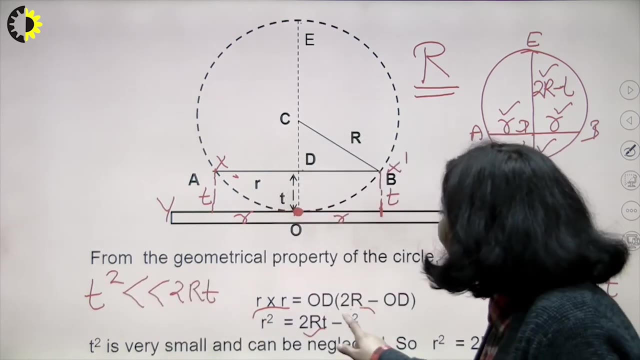 going to get here. you are going to get 2rt minus t square, so r square is 2rt minus t square and you know that radius of curvature is very large and that thickness of air film is very small. it means this factor t square. it is very, very small with respect to 2rt, so this can be neglected. 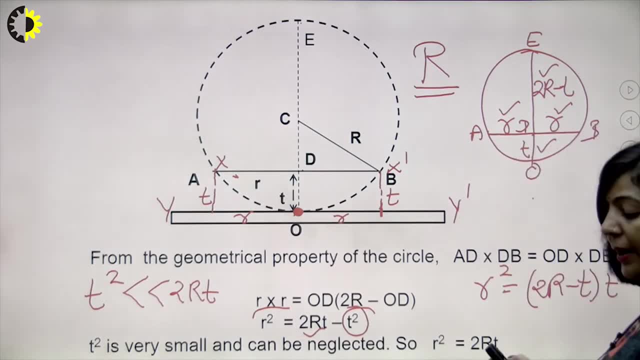 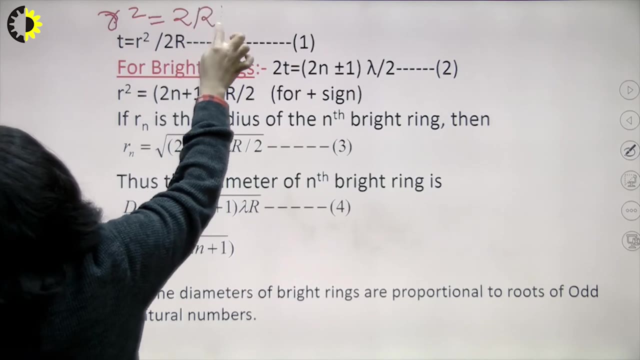 with respect to 2rt. so what will be the value of r square then? it means, now this t is r in square upon from here. what is the value of t? this r is r, square is 2rt, so we have to find t from here. 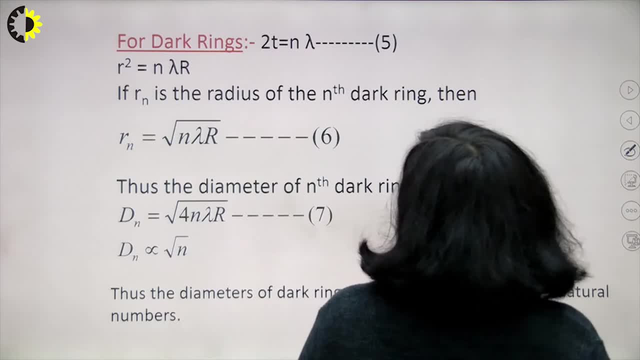 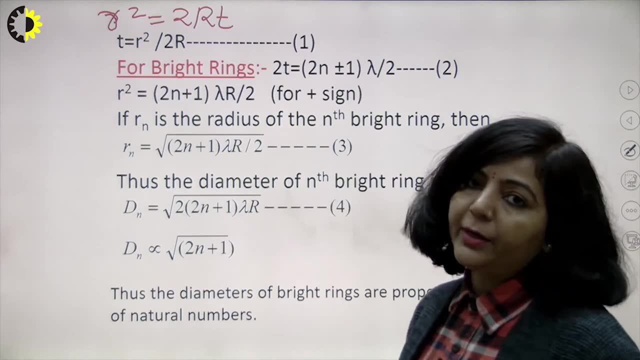 so from here, t is equal to r square upon 2r. sorry, r square upon 2r. this is your equation number one. now, using this thickness of air film, we will find a condition of maxima and minima. so for bright ring, you have what is the condition of maxima, this equation number. 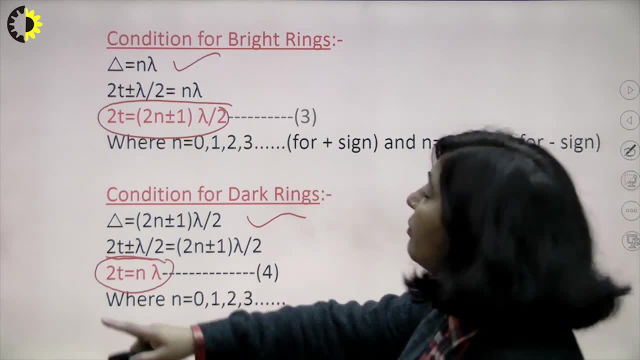 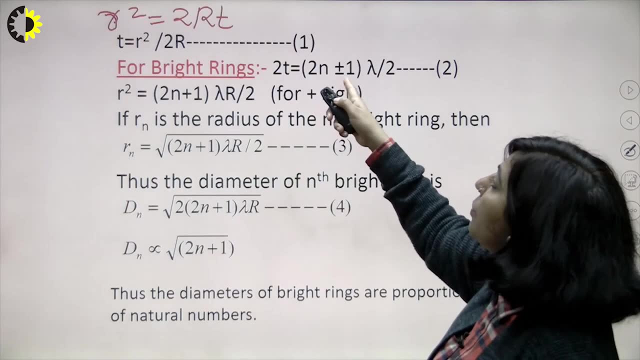 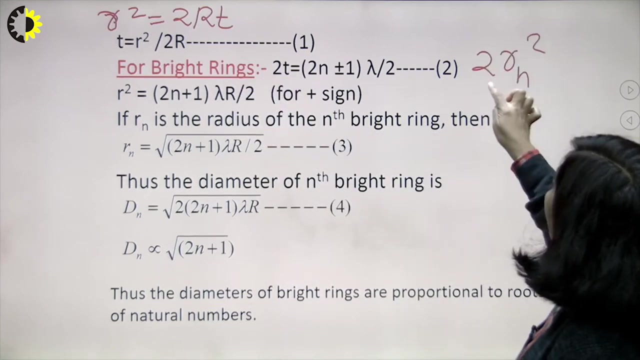 3 represents the condition of maxima. now i am substituting the value of t in this equation. so if you will substitute this t here, then what you are going to get 2 t is equal to 2 n plus minus 1 lambda by 2. instead of t we will replace this t with r n square upon 2 r, so this is equal. 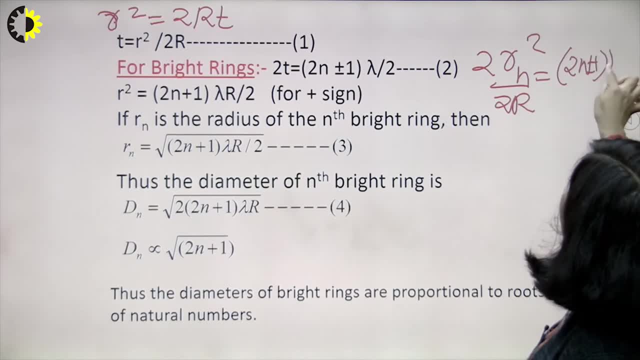 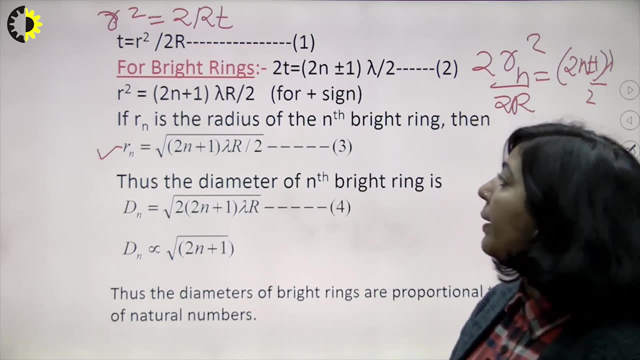 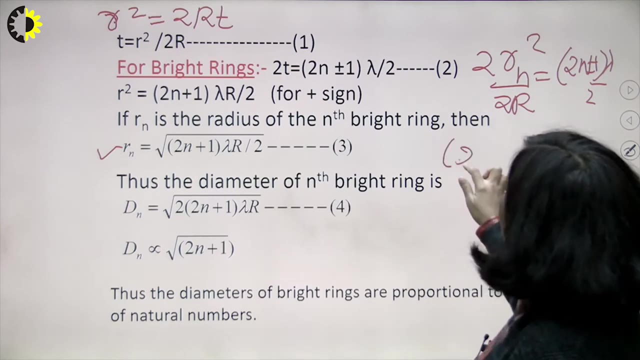 to 2 n plus minus 1 lambda by 2. so after substituting and simplifying, we are getting the value of r n, which is equal to this under root: 2 n plus minus 1. you can take 2 and plus 1. you can take 2 and minus 1, but the only difference is if you are considering 2 at 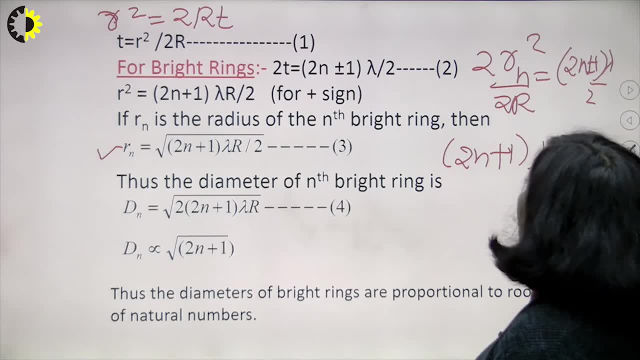 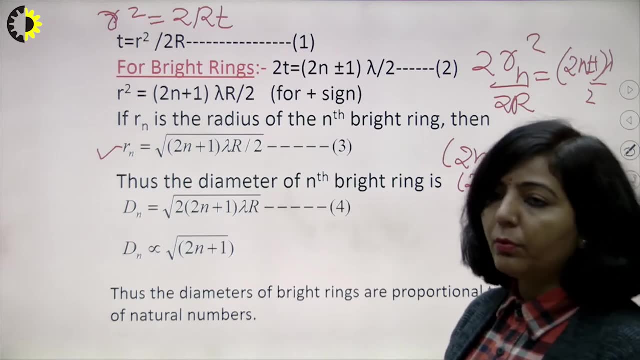 2 and plus 1, then n is going to start from 0, and if you are taking 2 and minus 1, then n is going to start from 1. that is the only difference. so it is up to you what you are going to decide. 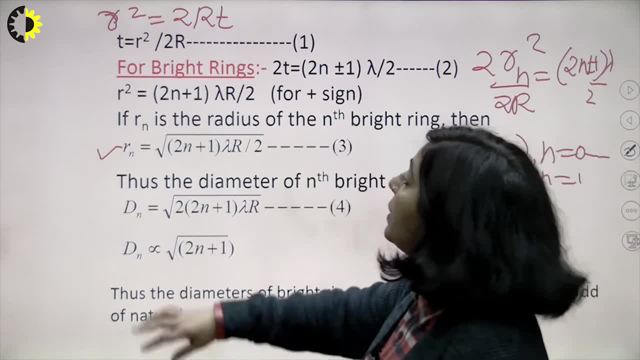 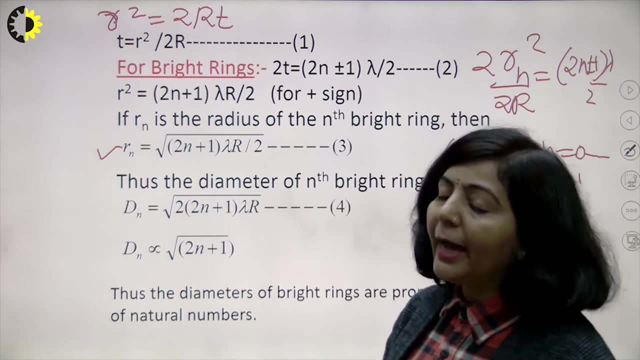 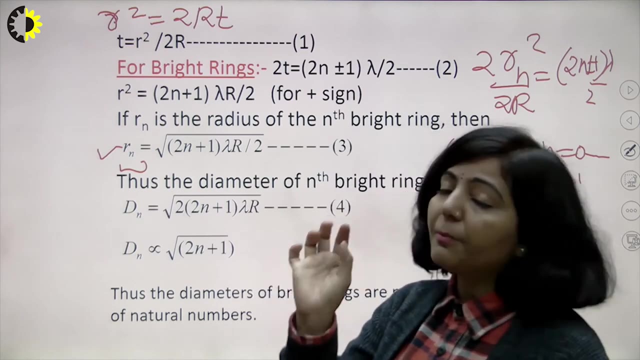 so if we are deciding this 2 and plus 1 factor, then this r? n is equal to this. so if you have radius of nth bright ring, you can find the radius of n sorry diameter of nth dark ring, sorry bright ring. so this radius r n equation number 3, that is representing the radius, so the diameter will be. 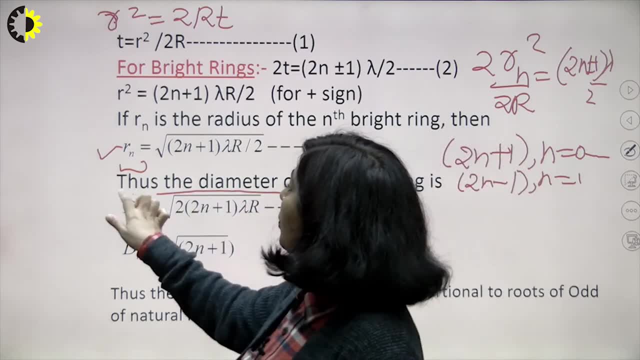 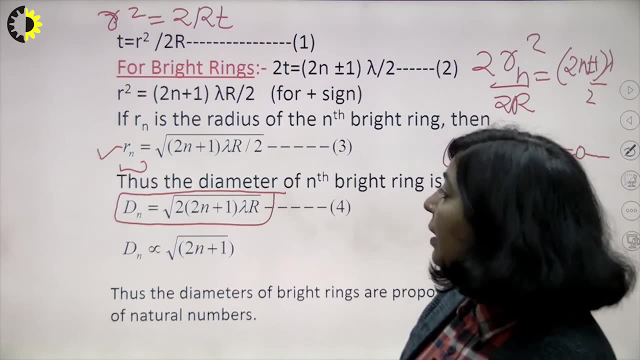 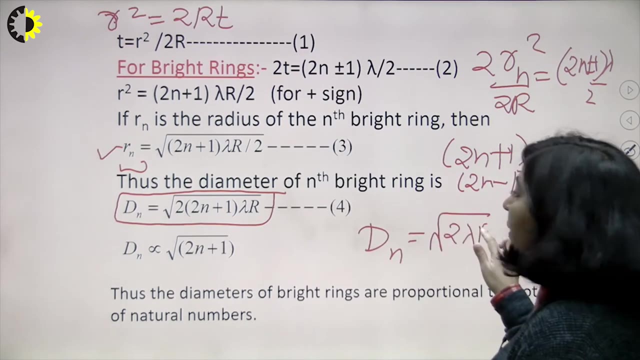 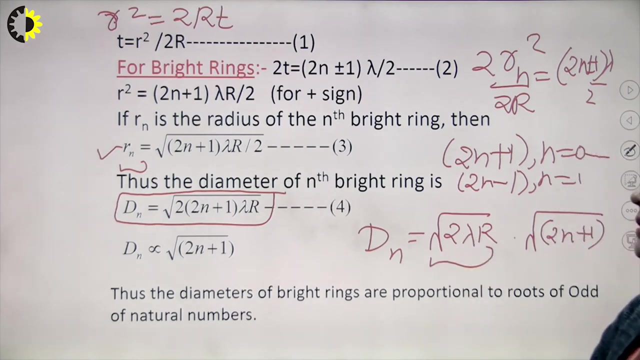 twice of this. so the diameter is simply under root 2 into 2n plus 1 lambda r. so this is diameter of nth bright ring. uh, and if you will see this equation number four carefully, we can write this as under root 2 lambda r into under root 2 and plus 1. so if you will see this, then this particular factor, this entire, 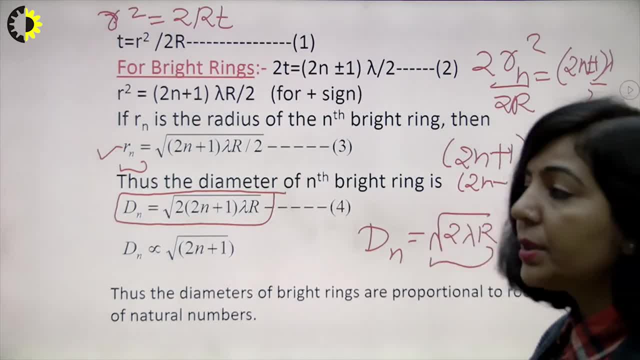 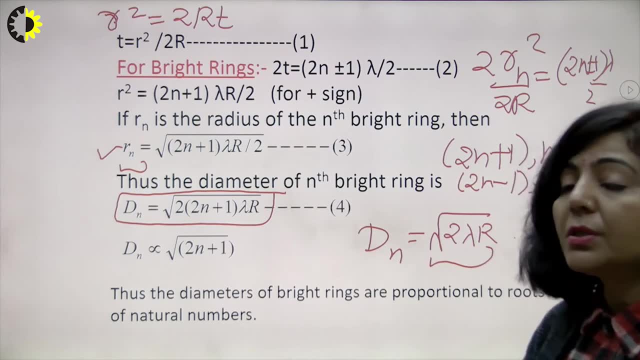 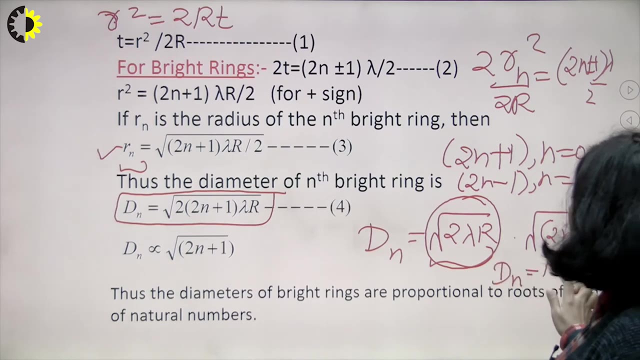 factor is constant. uh, root 2, that is constant. lambda is the wavelength of that monochromatic source of light. that is also constant. capital r, that is radius of curvature, it is again constant. it means this entire factor is constant. and if you are representing that constant with k, then dn is equal to k into root 2n plus 1, so i can say that dn diameter of nth bright. 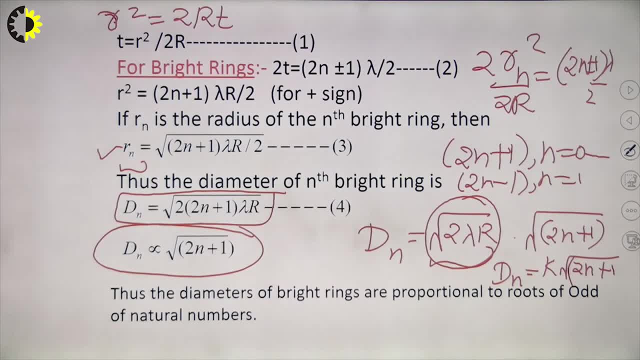 ring. it is proportional to square root of 2n plus 1 and you know n is going to start from 0. if n is taking 0 value, then it will give you root 1 it is taking. if it is taking 1 value, then it will. 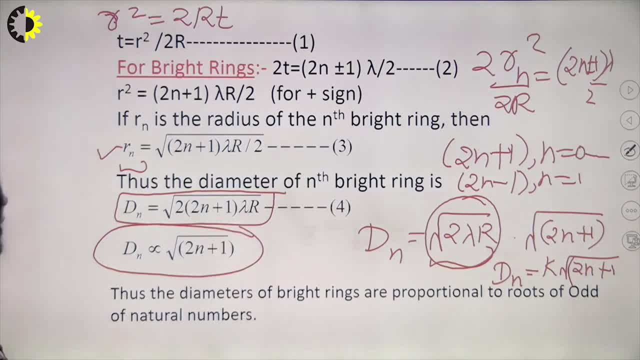 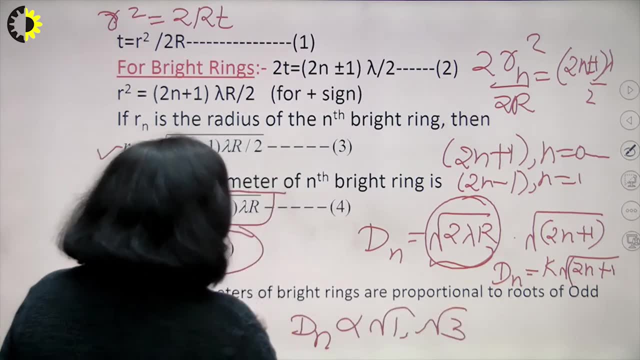 be root 3, next will be root 5, next will be root 7.. so what is the conclusion? the conclusion is that the diameter of bright rings that is proportional to uh. it is like this: uh, it is proportional to what is this proportional to square root of? 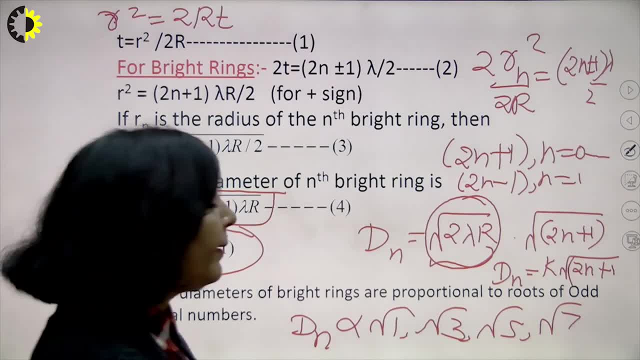 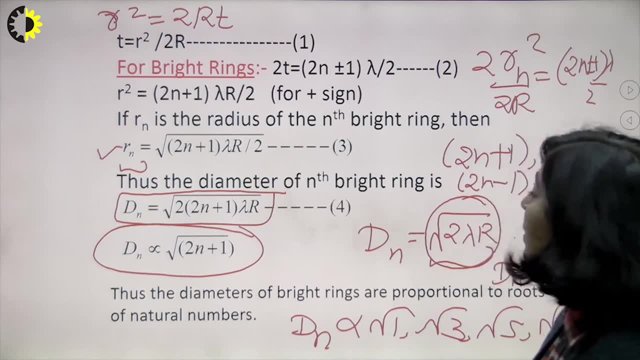 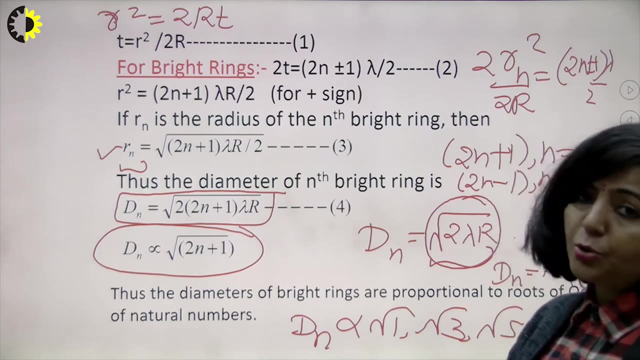 odd natural number. if you will substitute first value of n, then it is: dn is proportional to root 1. next value, dn is proportional to root 3, next is root 5, next is root 7.. so the conclusion is: the diameters of bright rings are proportional to square root of square root of odd natural. 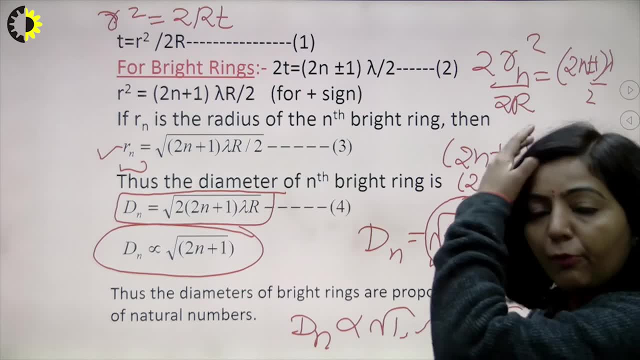 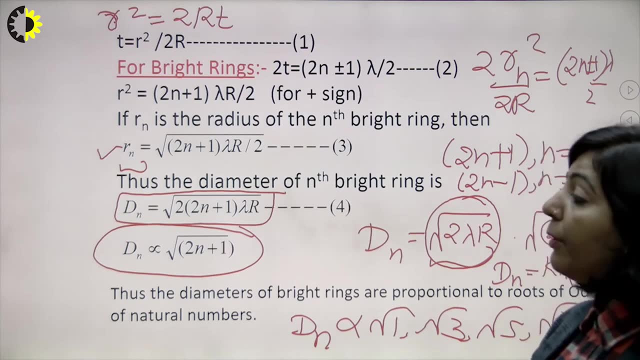 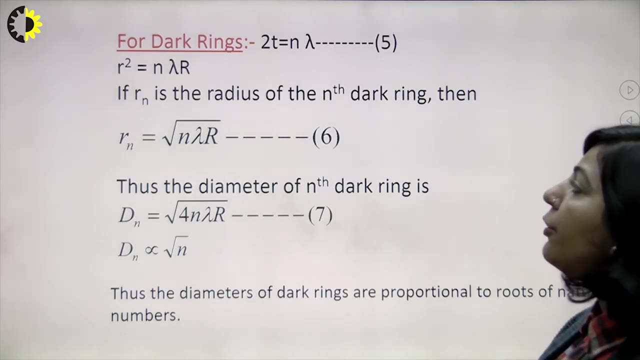 numbers. but this is the case of reflective system. in reflected system, you can say that dn is equal to root 2n plus 1.. so this is for bright ring. now, similarly, we are going to simplify it for dark rings. so for dark rings, you know, this is a condition of minima, or condition of dark rings. 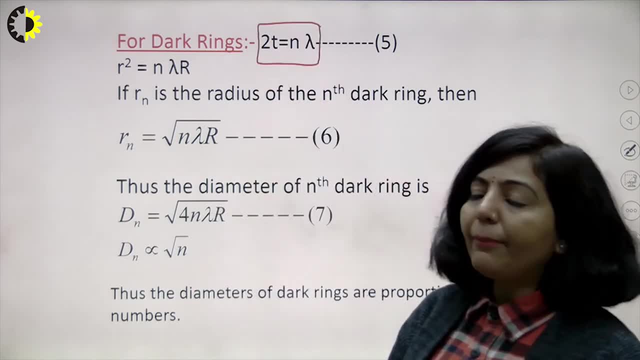 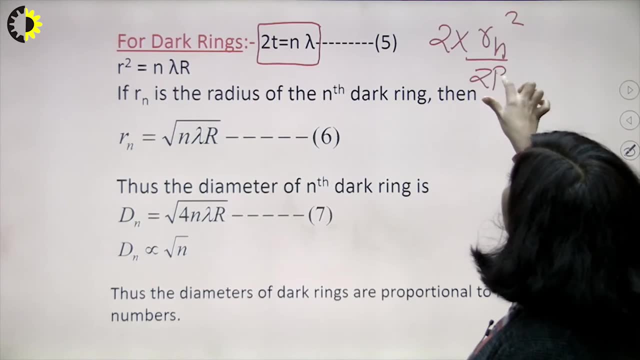 the 2t is equal to n lambda and you know you have to substitute the value of t here, and this t is rn square upon 2r. so if you will substitute t as rn square upon 2r, what you are going to get you? 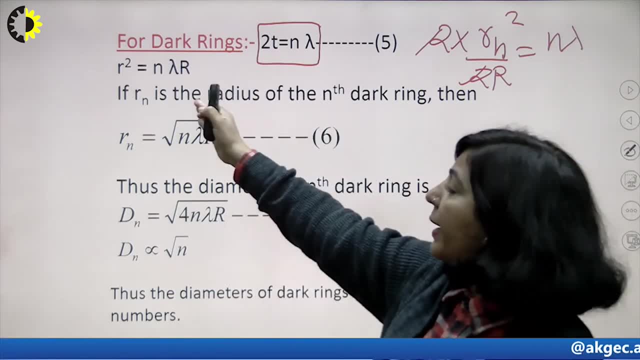 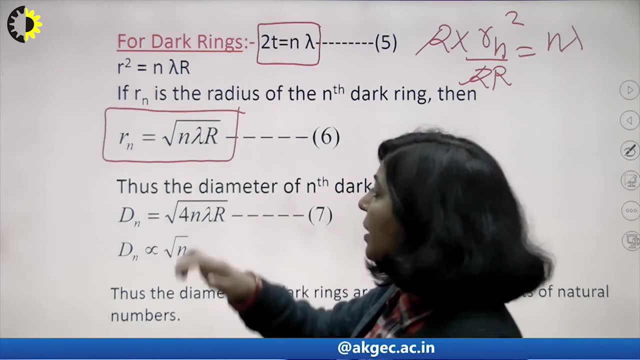 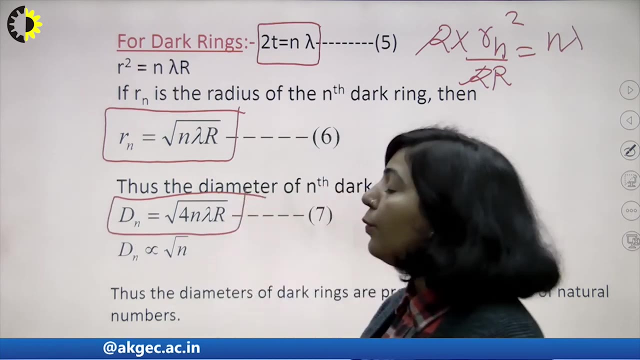 as n lambda r. so that is the method, how you are getting this r square as n lambda r. so what will be rn? it will be under root n lambda r. so if this is the radius, you can easily find the diameter. so diameter is square root of uh under root 4 and square root of 4 and lambda r. so if you will see, 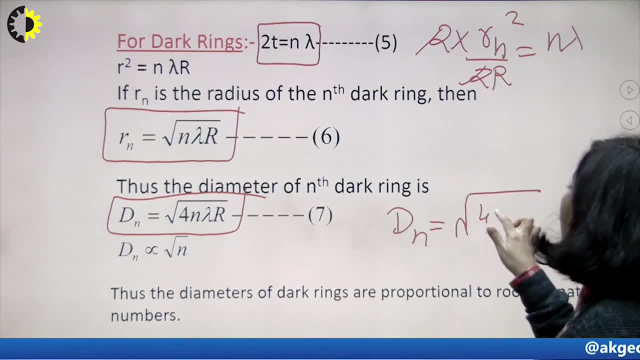 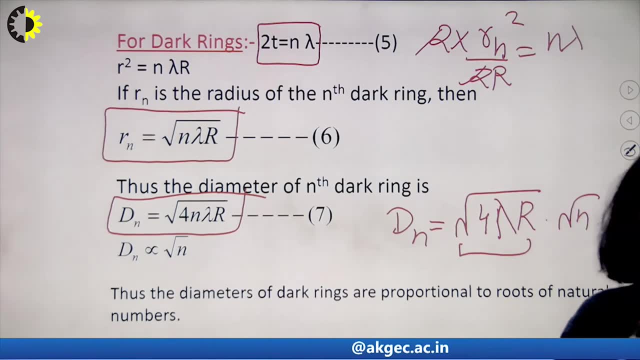 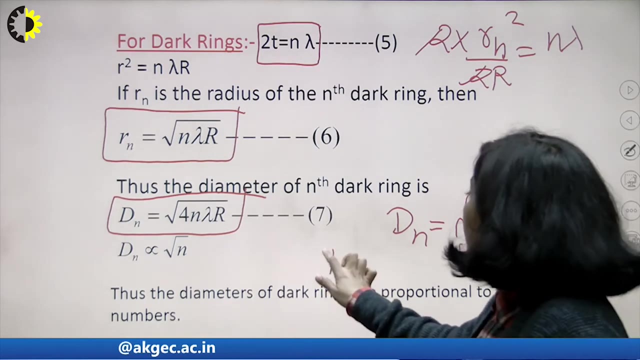 this equation, number 7, carefully. you can write it as: under root 4, lambda r into root n and you can see that this particular factor, square root of 4, is constant. lambda is constant. radius of curvature: that is again constant. it means the n. the conclusion is that dn is. i am taking this. 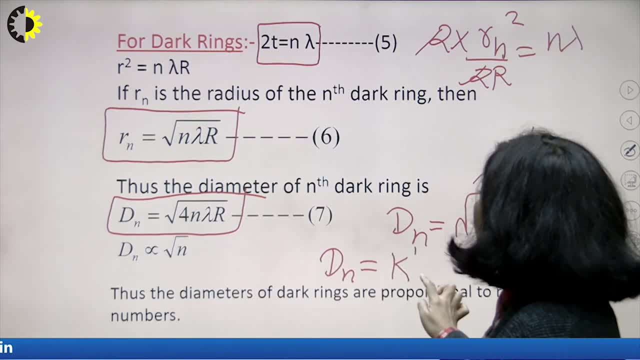 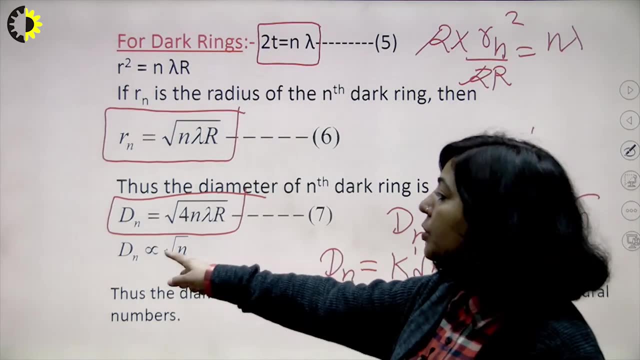 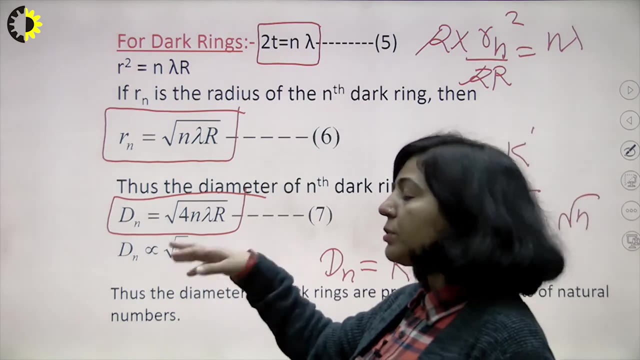 constant as k dash. so i can write dn: is k dash into root n. so the conclusion is that the diameter of this diameter of dark rings is proportional to square root of natural number and the diameter of dark rings are proportional to root of natural number. so, as you know, n is going to start from. 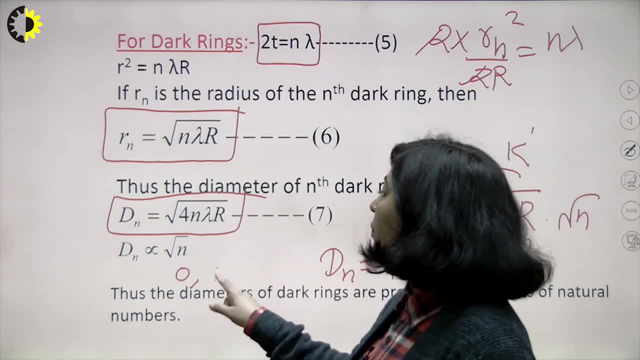 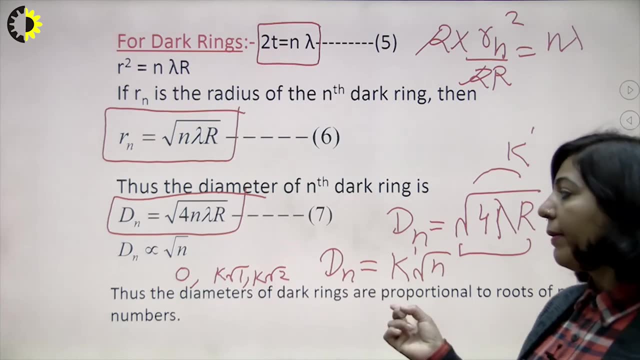 0. so the first value will be 0, next will be equal to k root 1, next will be equal to k root 2, next will be k root 3 and k root 4, and so on. that is why you are writing here. the diameter of dark rings are proportional to square root of. 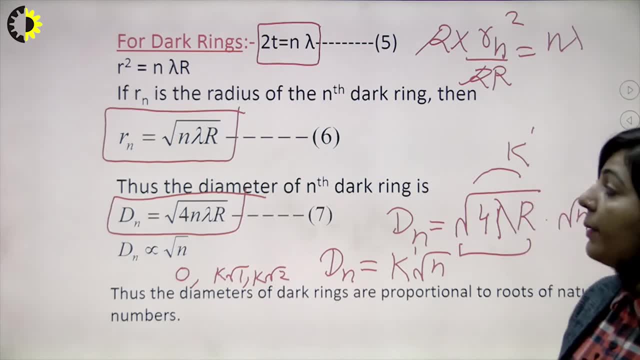 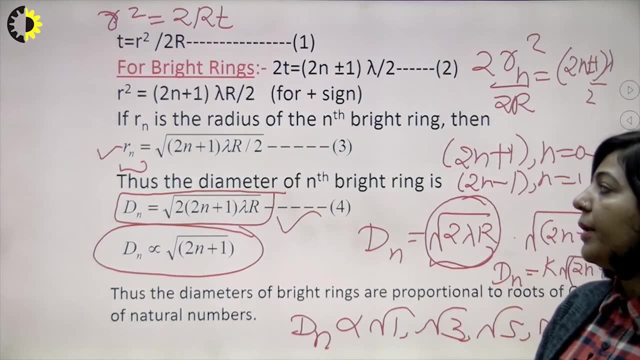 natural numbers. so these are the diameters of bright and dark rings. for bright ring, this one is the diameter under root 2 into 2 n plus 1 lambda by R, lambda into R, sorry- and the diameter of dark rings that is under root 4 and. 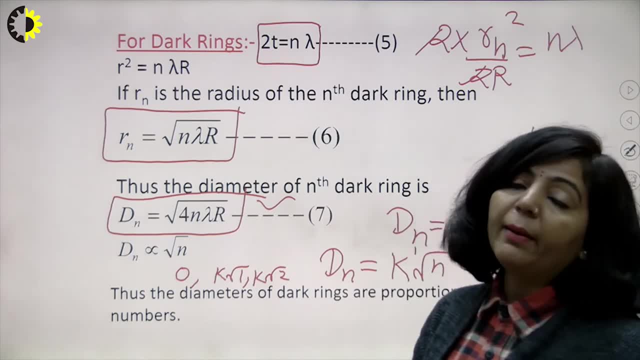 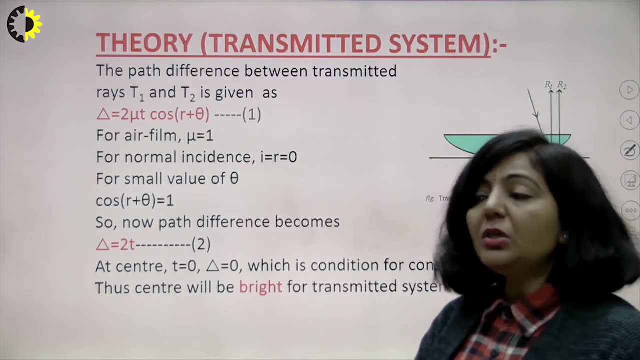 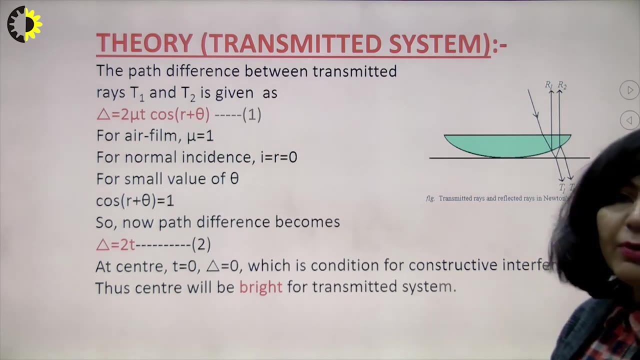 lambda R. so this is a matter to calculate diameter of bright and dark rings in reflected system. now, similarly, you can find the diameter of these bright and dark rings in transmitted system. so, in order to find that you know, in case of transmitted rays, if we are taking a bed sheet film, why I am saying. 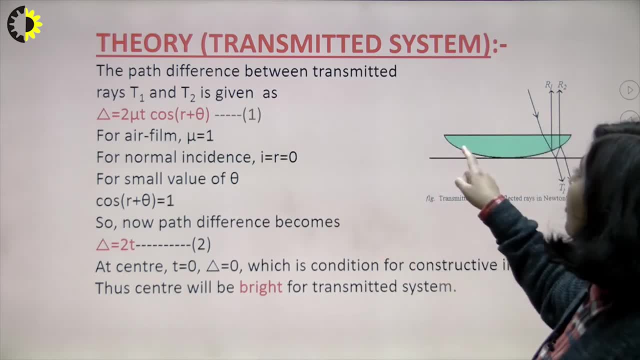 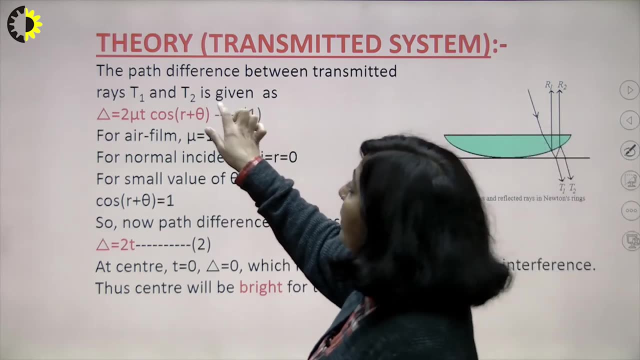 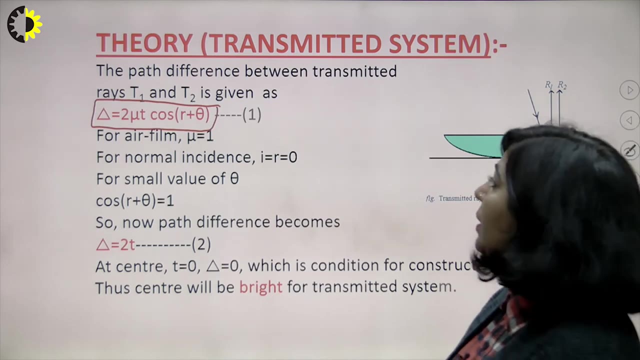 we are having a wedge shape film because between this play-doh convex lens and glass plate we are having that air film, bed shade film and for bed shade film in transmitted system. this equation number one, that represents the part difference. now, again, using the same logic that r, light will incident normally. so r is zero. so if r is zero, then cos. 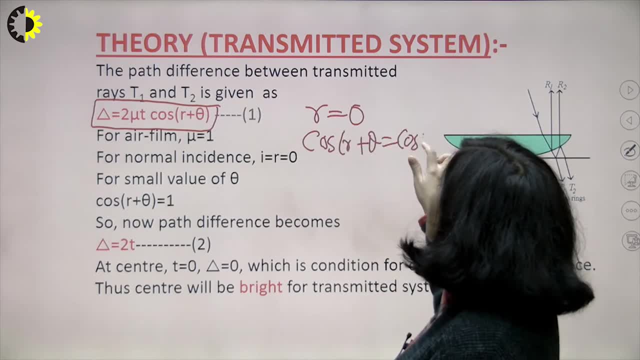 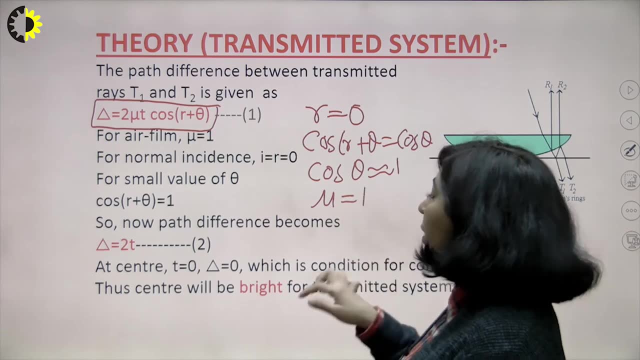 r plus theta, that will give you cos theta. and since theta is very small, so for small value of theta, cos theta is approximately one and since you are having a air film between plano convex lens and glass plate, so this mu is equal to one. so because of this reason, the part 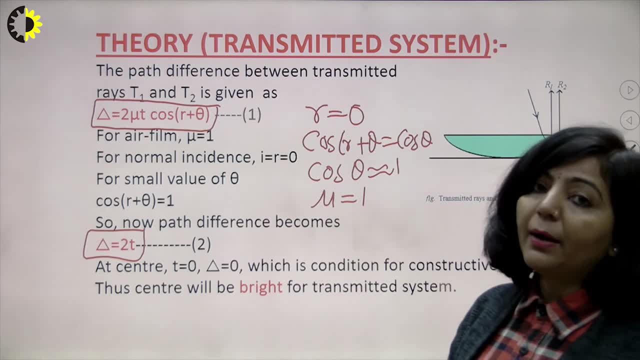 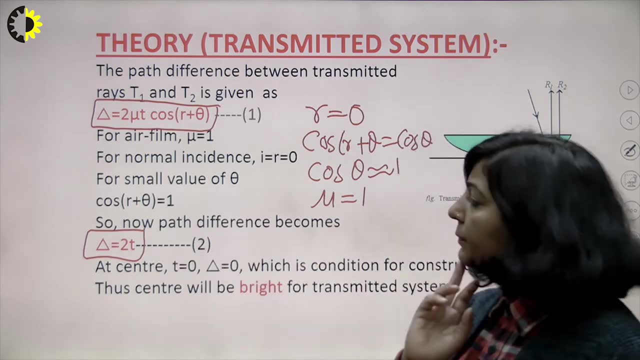 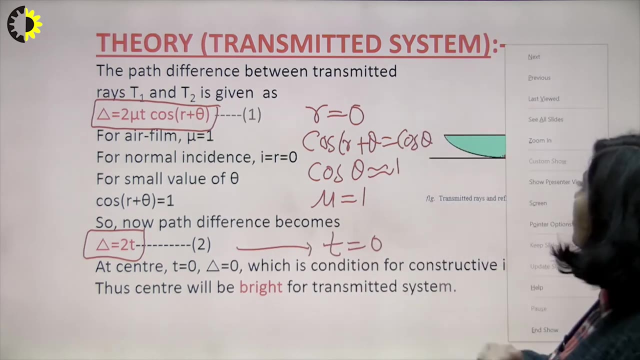 difference is only equal to 2 t. so this is the power difference in your transmitted system. now, according to this relationship, if you will see it carefully, at the point of contact, at the point of contact, this t is zero. means, at this position, at this point of contact, 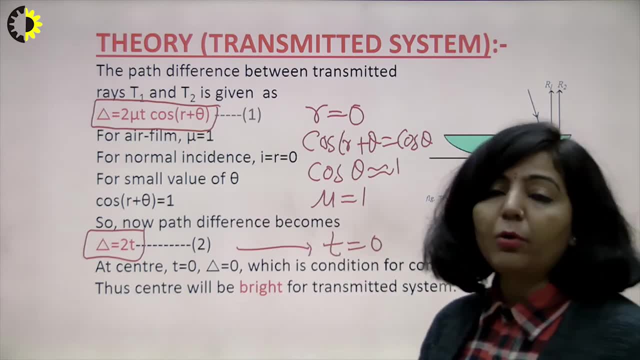 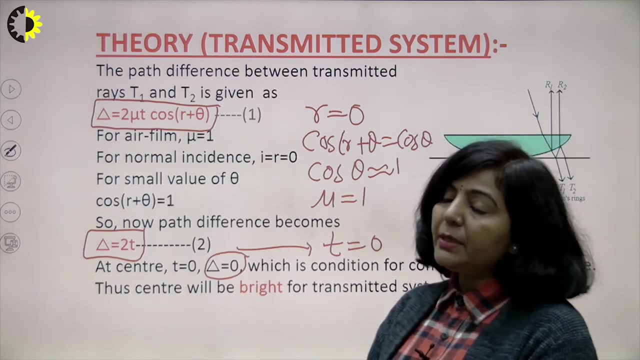 when t is zero and scattergun is at two. now that must beM is equal to mal. highlight: vincia is 0, then your delta and delta, or you can say part difference. that comes out to be 0 and you know the part difference, 0. that is the condition of maxima. it means in transmitted system, at the 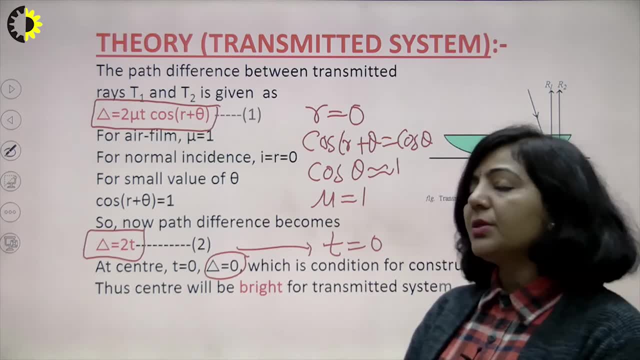 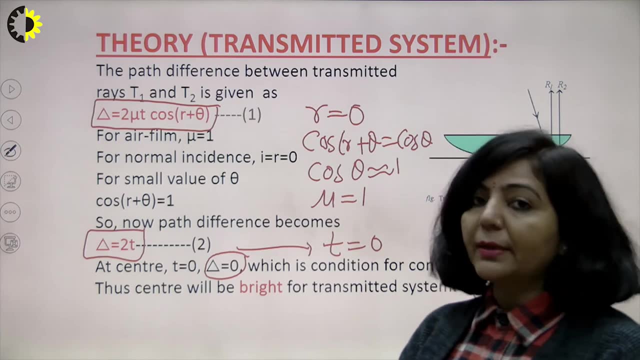 center we are going to get a bright ring, whereas in reflective system, as we have discussed since at the center, the part difference will be lambda by 2 or multiple of lambda by 2. that is the condition of minima. so that was the reason: in reflective system you were getting a dark ring. 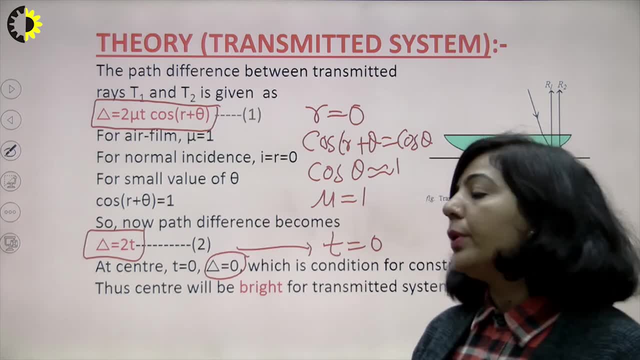 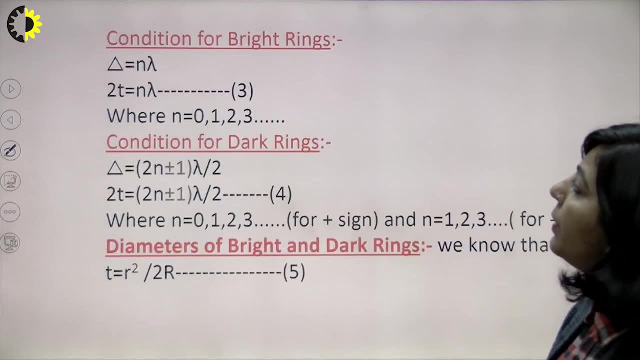 at the center, whereas in transmitted, since the part difference is 0 here. so you are getting a bright ring at the center. so now, using this part difference, we will find the condition of maxima and minima. so for maxima, you know, part difference should be n lambda. so part difference. 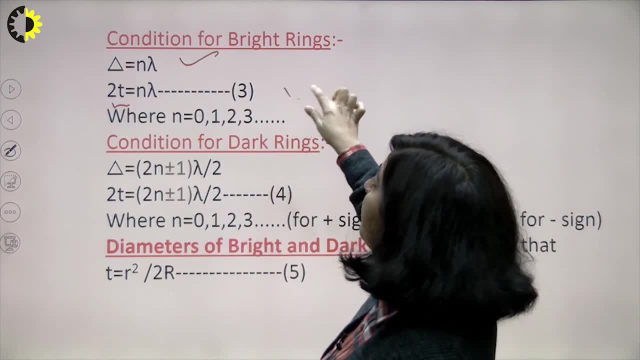 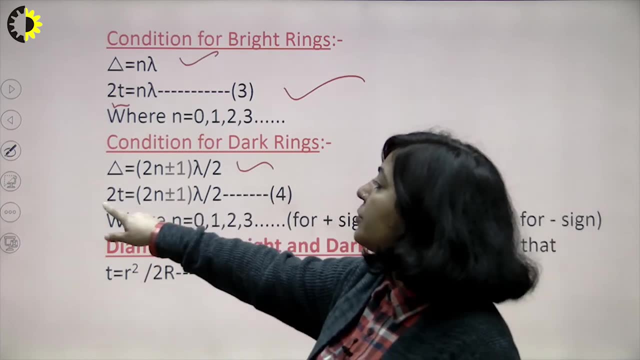 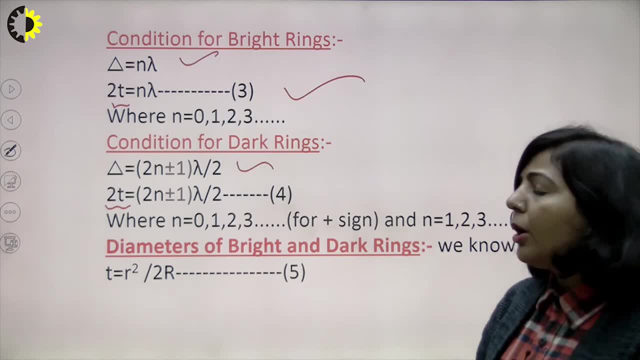 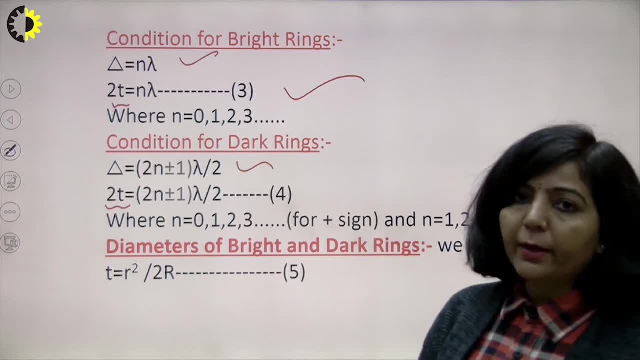 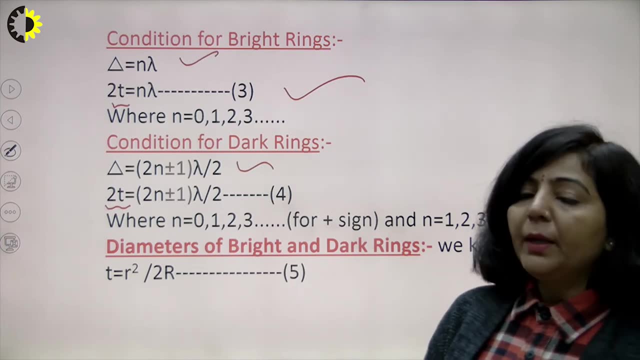 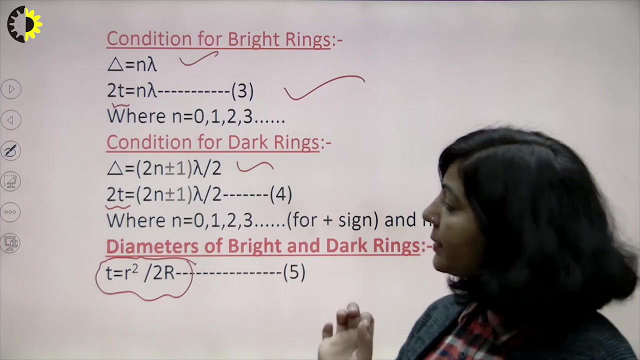 dark rings in transmitted system. so you know how to find it. in order to find the that diameter of bright or dark rings, first you have to find the thickness of air film. and you know the thickness of air film. the general expression for thickness of air film is r square upon 2r. so using this, 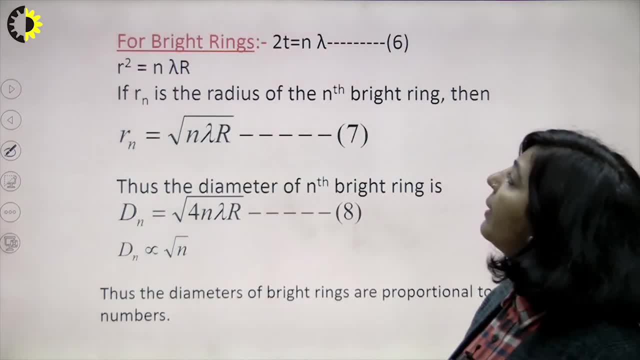 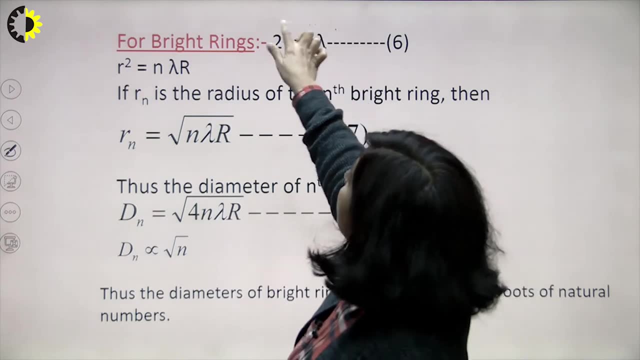 thickness. now we will decide the condition of maxima and minima. so, for maxima, since you are having this condition, what is the condition of maxima and minima? so for maxima, since you are having this condition, what is the condition for maxima? 2t equal to n lambda, so 2t is equal to n. 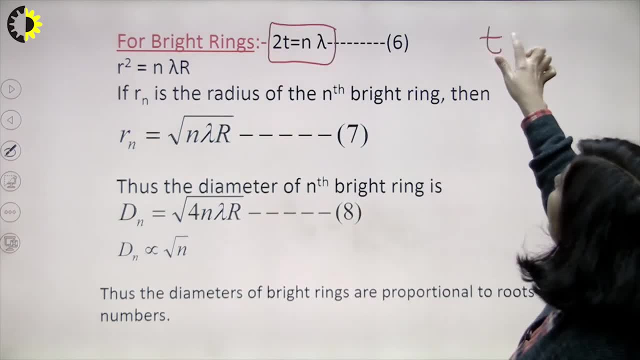 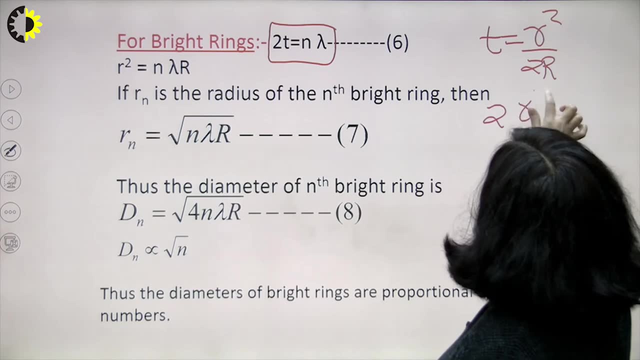 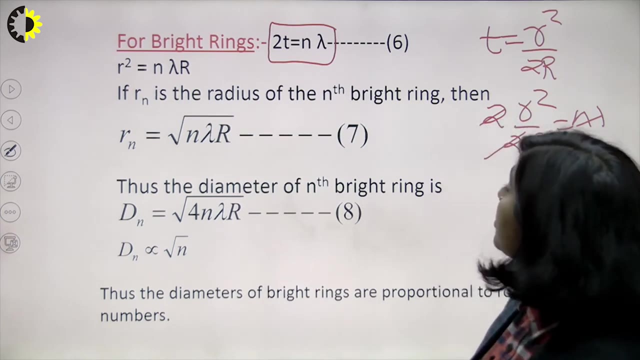 lambda is the condition of maxima and in this condition we are going to substitute t as r square upon 2r. so if you will substitute t as r square upon 2r, it will be 2. r square upon 2r is equal to n lambda. so what is the formula for r square? or you can say rn square, it is your. 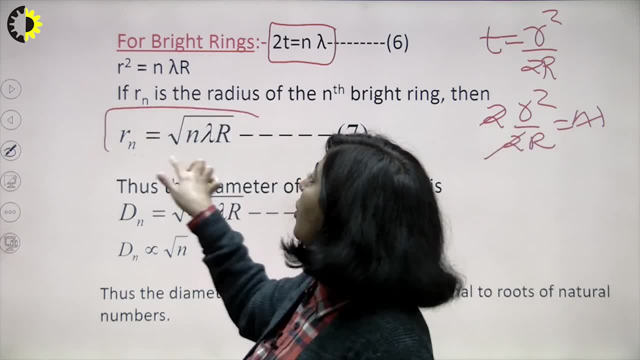 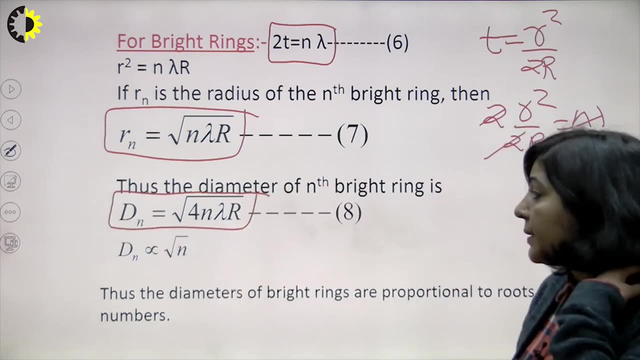 n lambda r, so rn is this square root of uh n lambda r, so dn will be equal to squashy square root of 4 and lambda r. this is uh the diameter. uh, sorry, this is the diameter of your nth bright ring and, using the same logic, that dn is proportional to square root of n. 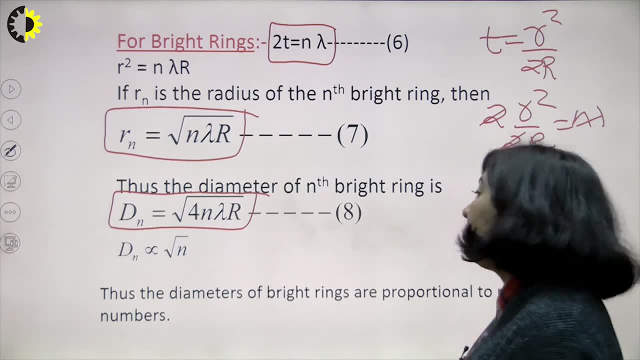 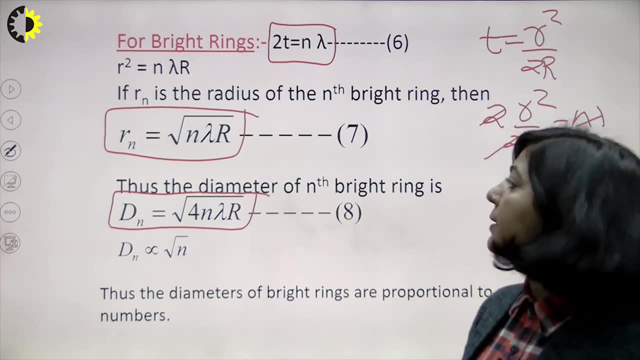 it means diameter of bright rings in transmitted system is proportional to square root of natural numbers, which is, uh, just opposite to your reflected system. and for dark rings, since you know this is the condition, 2t is equal to 2n plus minus 2t, and square root of 4 is白 ring, so 2n is. 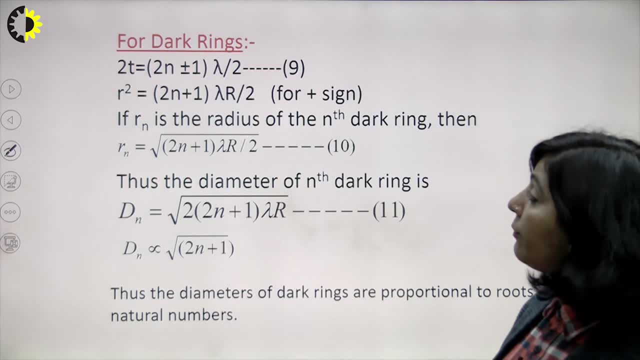 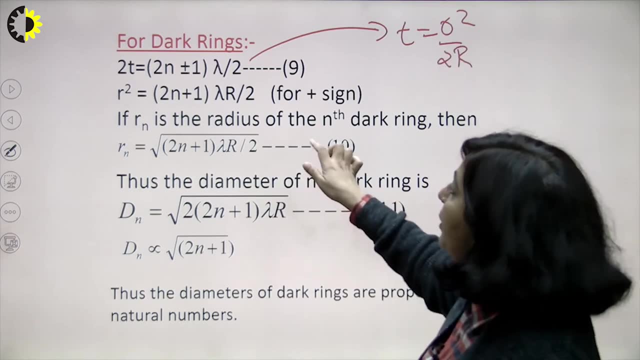 proportional to square root of 4. it means that the diameter of the transmitted system is proportional to square minus 1 lambda by 2.. So what we have to do, We have to substitute here the value of t, which is equal to r square upon 2r. After substitution and simplifying, you are getting this equation number. 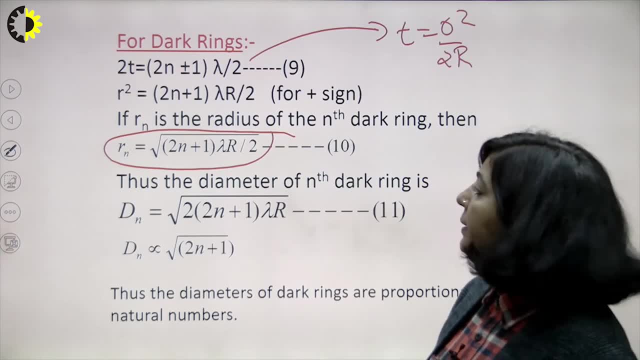 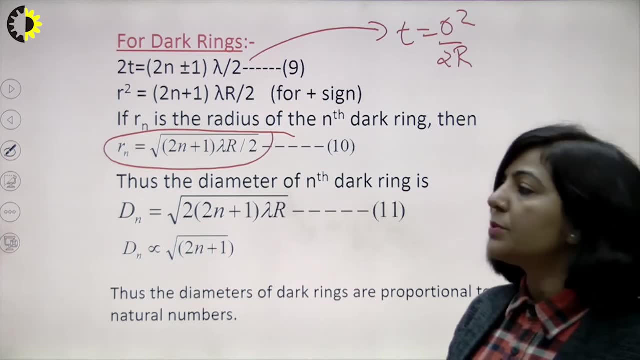 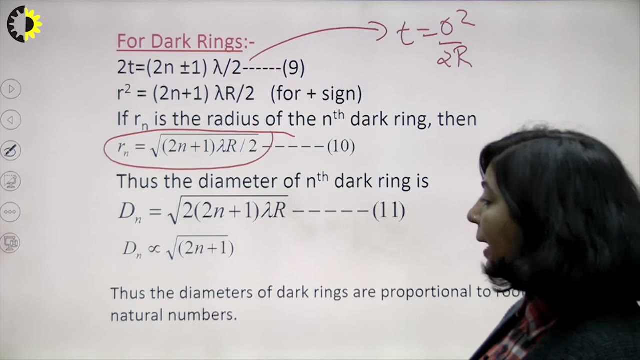 10, and if equation number 10 is the radius, then the diameter will be simply that will be given by equation number 11. dn is equal to square root of 2 into 2n plus 1 lambda r. Again the same conclusion: that dn is proportional to square root of 2n plus 1 means diameter of dark rings. 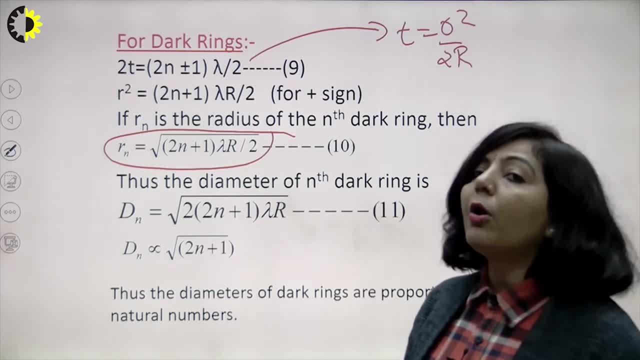 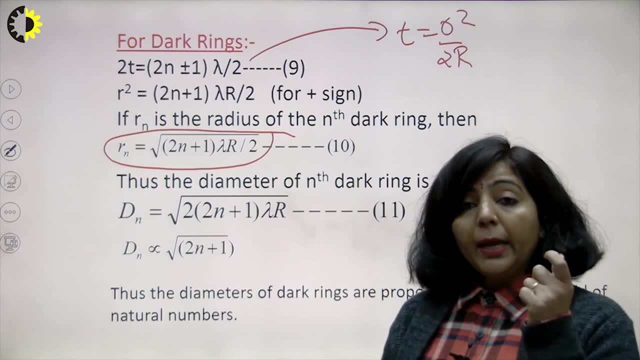 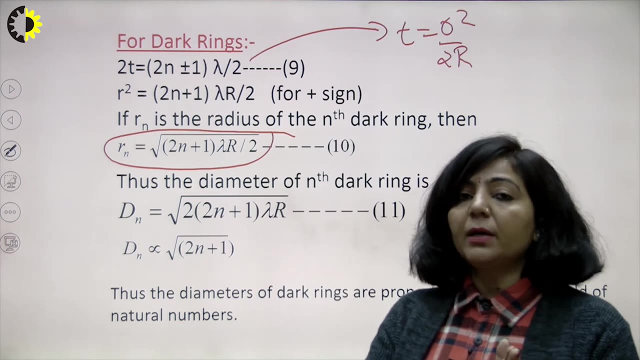 in transmitted system is proportional to square root of all natural numbers, Means the results of transmitted system are just opposite to the results of reflector system. In reflected the center is dark, whereas in transmitted center is bright. In reflector system the condition of maxima, or diameter of maxima, is square root of 2 into 2n plus 1 lambda by r, whereas this condition 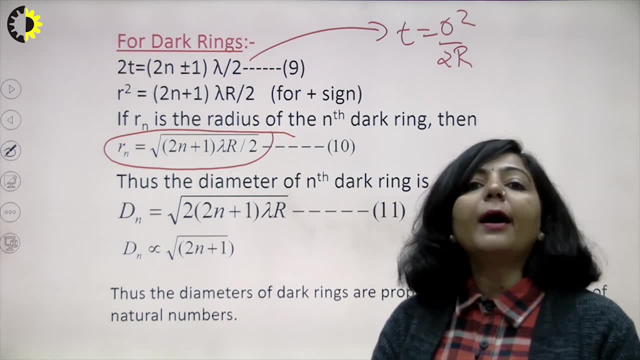 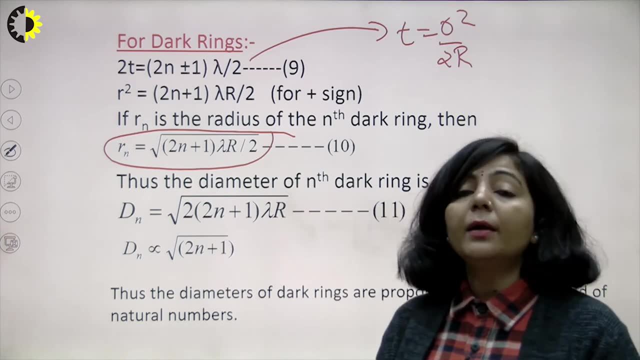 same condition or same diameter is a diameter for nn dark ring in transmitted. In case of reflected, the diameter of dark ring is square root of 4n lambda r and this square root of 4n lambda r, that is the diameter of nth bright ring in transmitted. So these systems, that is,